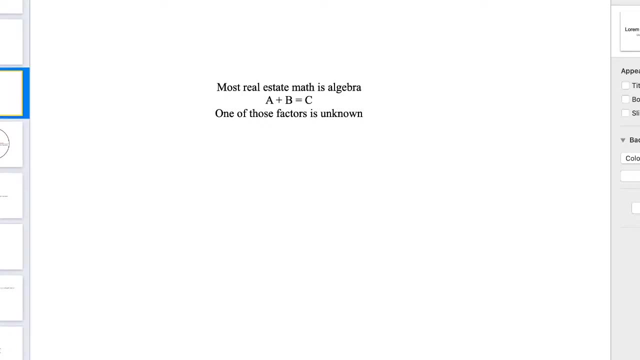 call. This is for our premium members. Okay, So we're doing math today. Um, I know a lot of you guys freak out about math and drives me nuts when you do, cause I don't want you guys freaking out about it. Math is not a large portion of your exam. It's a small portion And a lot of time. 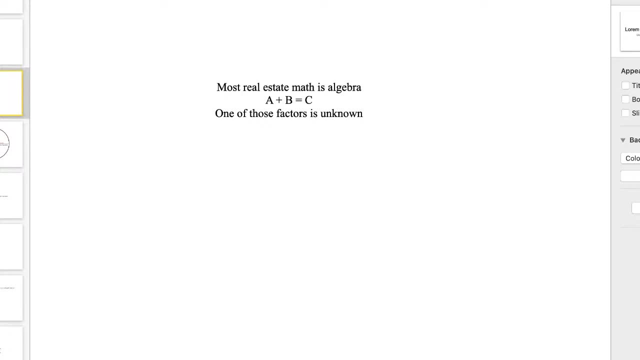 people focus on what scares them the most. Anybody do that. You focus on the things that give you the most anxiety, when really you should be focusing on the things that you are strong at. Okay, You should not be spending all your time focusing on the thing that gives you the 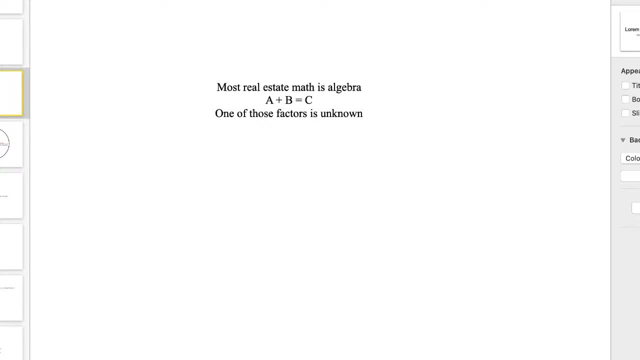 most anxiety. That'll kill your confidence, It'll be discouraging And also it'll take up a lot of time and energy that could be more put towards things that you could do very well, like real property, um, personal property, all that kind of stuff. So when I hear people say I failed because 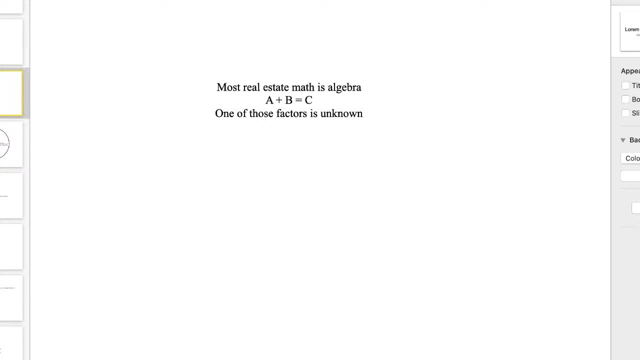 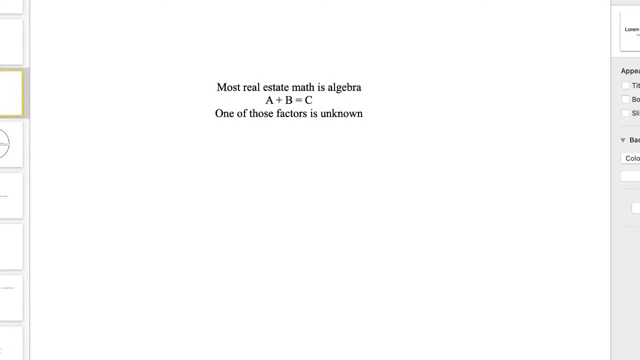 let what scares you take away from you learning everything you need to know for to pass the exam and get your real estate license. All right, Everybody got it: Yes, Yes or no, Yes or no. So I often so. Adrian and I teach the math a different approach. That's why he does it, and 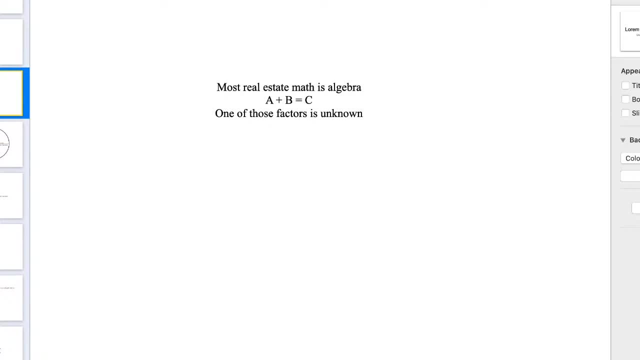 I do it, which is great. I love that we kind of take a different angle at this. For me, when I teach math, what I did is much like I just told you about the exam. I approach math in the same way. 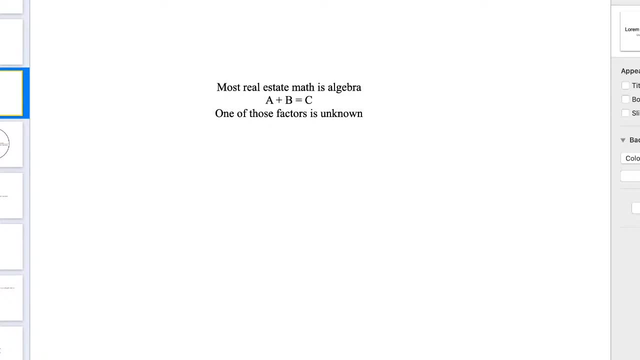 Let's say you have five math problems. Okay, I want to at least get two of those correct. One, I'm not sure, And the other two will just be a straight up guess. Okay, The other two would just be a straight up guess, you know, but I want to want to be scared of math as a whole. That's my. 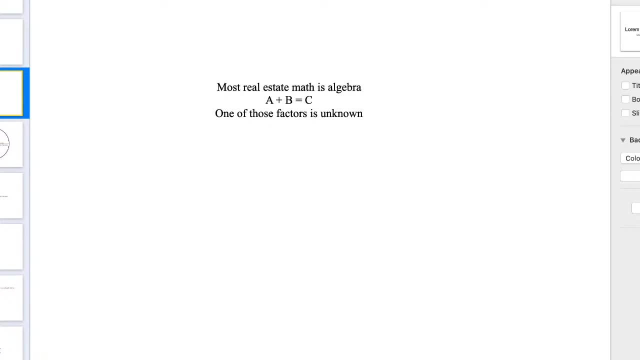 point. I don't want to sit there and just be like, Oh, there's a number, I'm scared of it. Okay, You guys should see it. I don't want to sit there and just be like, Oh, there's a number, I'm scared of it. 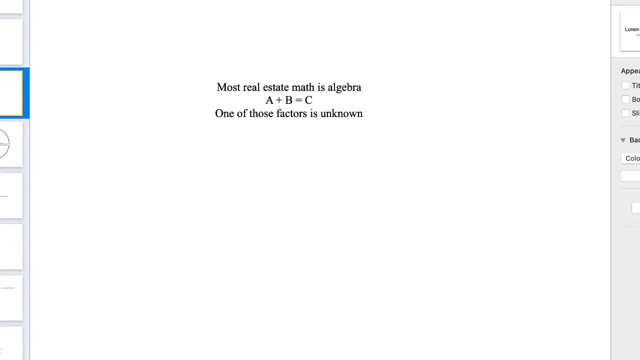 I don't want to sit there and just be like, Oh, there's a number, I'm scared of it. Okay, You guys should see certain words that make you say, Oh, I got this, This is no problem, No problem at all. So for 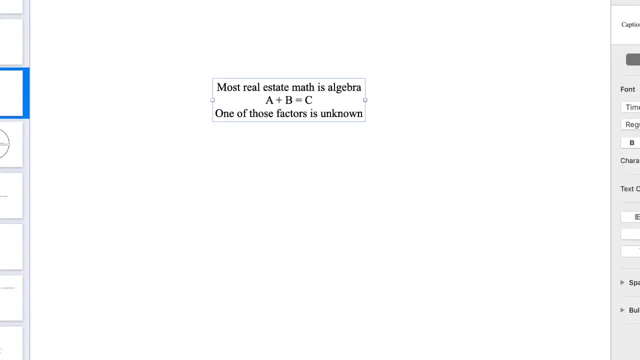 me. the two that you guys should absolutely be not scared of is one: commission problems. Okay, Anytime you see a commission problem, you should be all right. Now, part of as I say this is: I know you guys are scared of math and we break this down and you'll say: you know what This isn't. 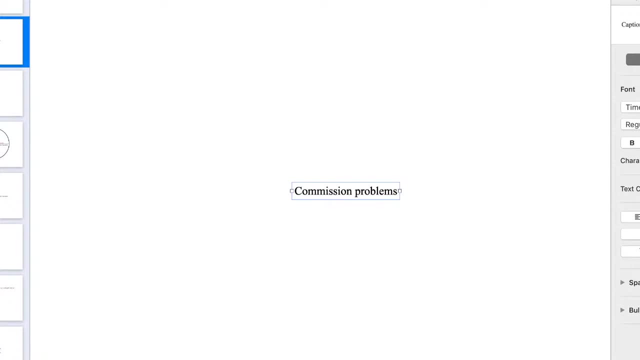 a mission problem. So the moment I saw on my exam, okay, I saw the word commission, I was like rock and roll, Okay. I was like ready to go commission, Okay. And percentage problems: Okay, You guys should know commission percentage and the rest is just basic algebra, basic algebra. And if you 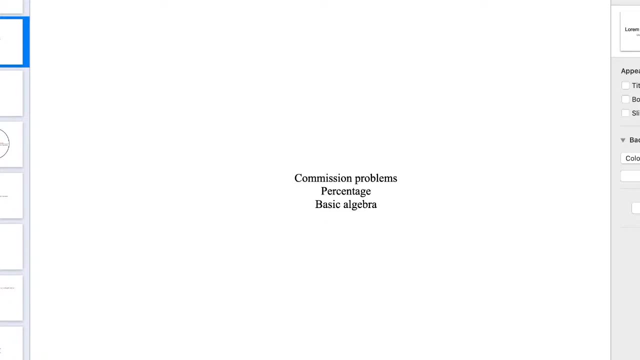 know those things. math is not hard. Aaliyah, don't say math is hard, It's not hard. If you guys focus on the math, that is easy, you'll be okay. Everybody got it. Much of these math webinars I find myself trying to make everybody relax. Okay, Um, you see, math you get. 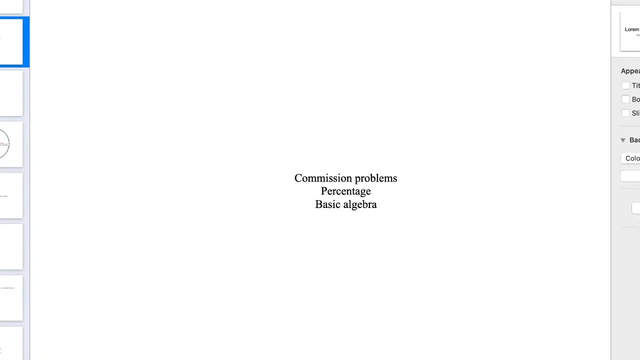 scared. but if you break down the math, say wait a minute, two or three of these, I know I could do without an issue. So my first piece of advice for you guys: make sure you know how to do commission in every way, shape and form one, because you're going to want to figure out how you get paid. 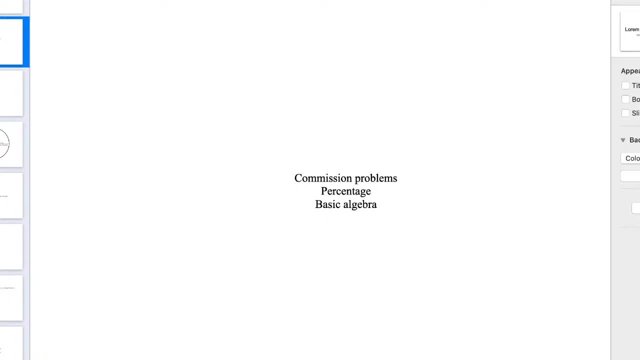 And then when you see math, you see commission. you'll be able to do it. I guarantee you're going to get a commission problem on your exam. That's basic. Everybody got it. I guarantee. I want to say that again. I guarantee. 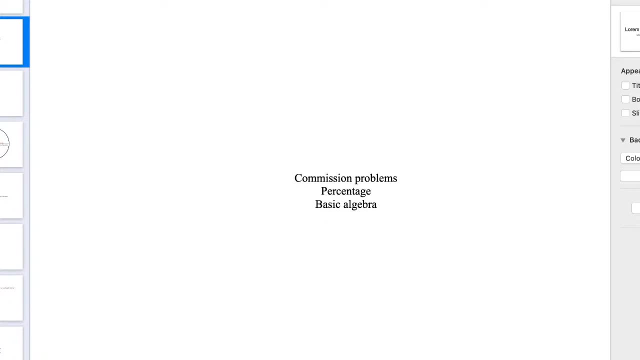 one of your math problems is going to be a commission problem. Okay, Is everybody got that? So right there. that ticks off some of the math. So math is small percentage. Now we just take that off. Okay, So math is basic algebra. Uh, most of the math you see on the real estate. 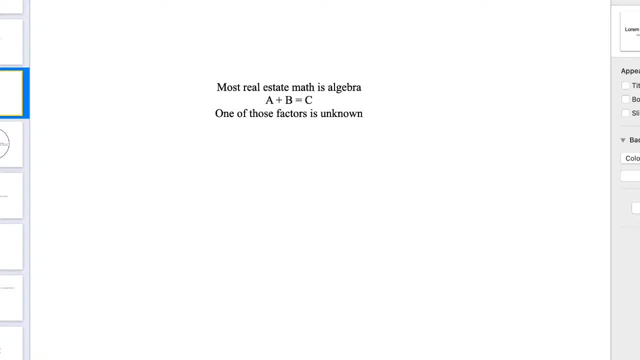 the exam is a plus B equals C. You figure out the, the, the unknown factor, All right. Or sometimes it's a times B equals C, but it's basic, Um, I'd say freshman year of high school algebra, or eighth. 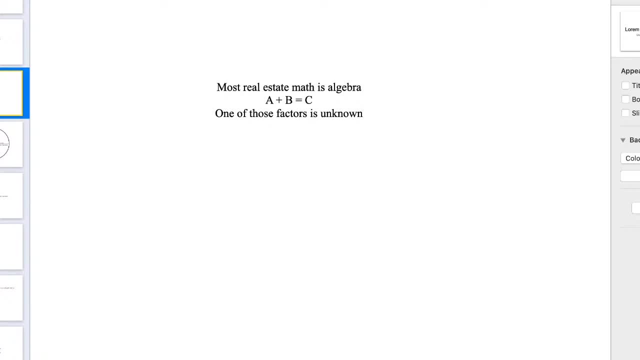 grade algebra. I don't know about you guys. Some of you guys see this T formula. Adrian, I don't love this, but if you guys do love it, this is what it looks like. Okay, Everybody see this on the board. 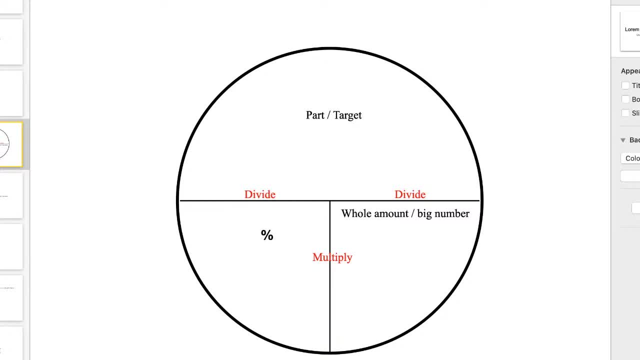 Okay, And you can write it down if you want. For a lot of us I think it just makes it unnecessarily cumbersome, but some people it helps them organize their thoughts. Okay, So you have this line here going across line up and down. You put the things in the different areas: divide, divide. 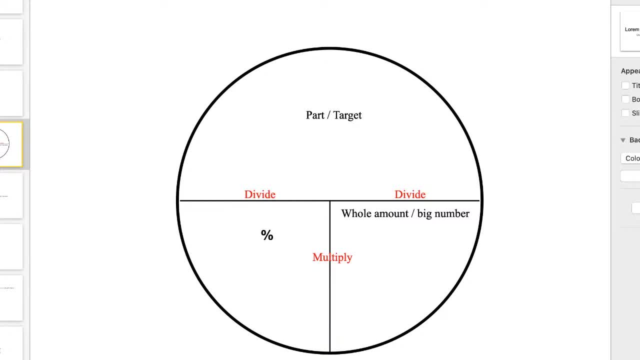 you go to here to here you're dividing, go from part to the percentage divide, part to the whole amount of divide. here and here you've got multiply. Okay, You put up top the part or the target number on the bottom left, the percentage, now the bottom right. 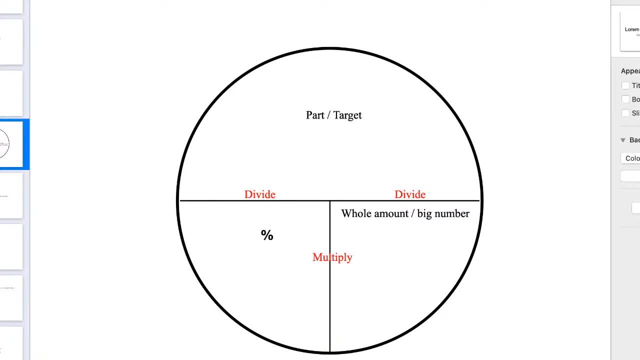 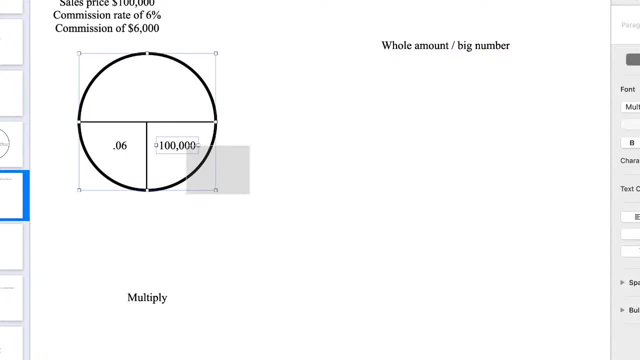 the whole big number, the big amount. Um, we will take a look at this in a little bit, but here, if you look at here, I'll give you an example of what we're talking about If we use this for a commission. 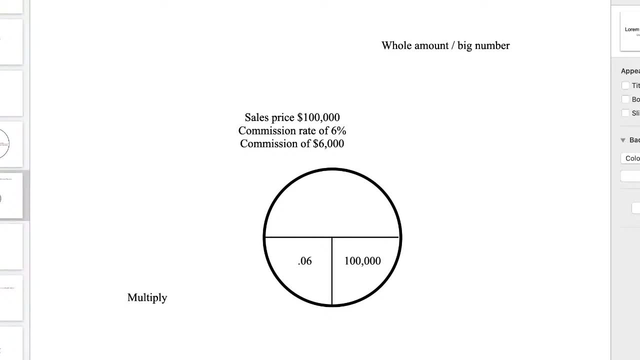 problem. everybody see this commission problem. All right, You would take the a hundred thousand is that's the big number. The percentage 6% is 0.06, right, Guys? what's 0.06 times a hundred thousand? What's 0.06 times a hundred thousand? What do you guys think it is? 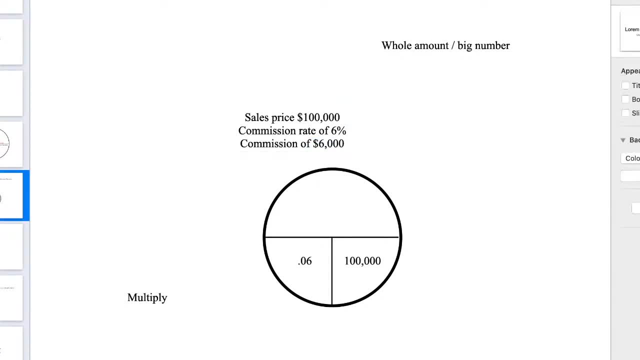 6,000 and the 6,000 would go right over there. Okay, Does everybody see that? Now, if you divided 6,000 by 0.06, you know you would get a hundred thousand. All right, Now that's that T formula. You guys could use it. You don't have to. it's just a way to organize your. 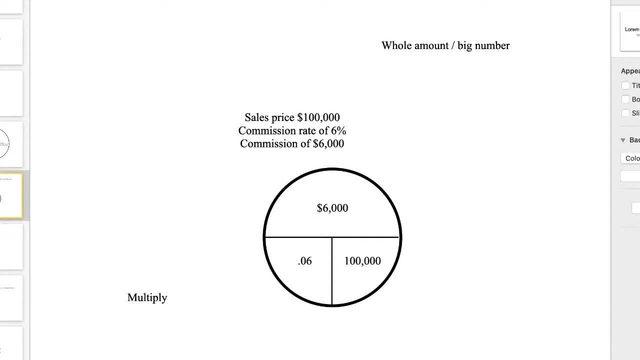 thoughts. I think it's just easier just to lay it out like a typical algebraic issue, but that's one way of doing it. Okay, everybody good. So when you hear the t formula, that's what they're talking about. 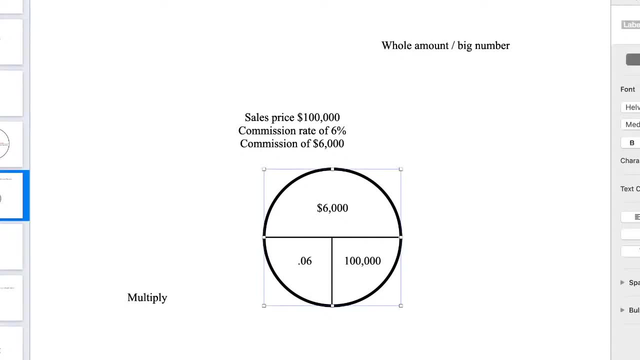 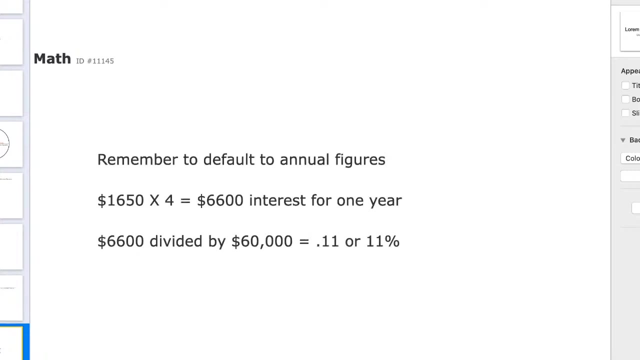 You don't really need the circle. You could do it without the little circle if you want. I just liked the circle. Okay, Let's do an actual problem here. All right, Let me see if I can find a nice commission problem. 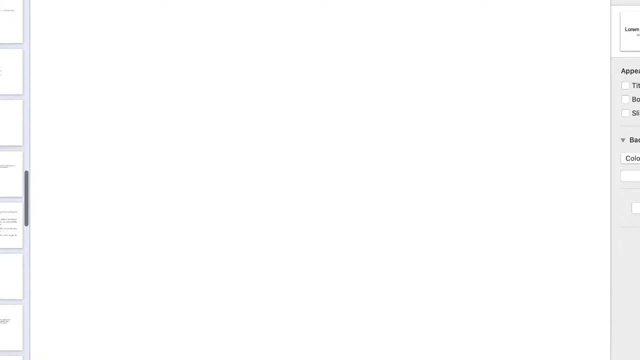 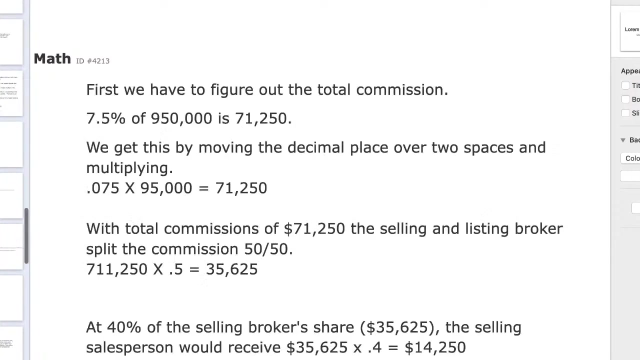 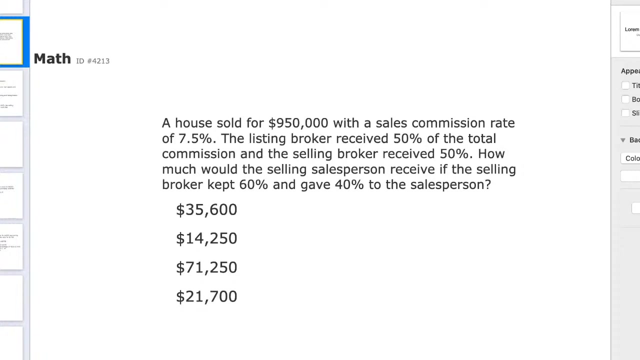 Coming You out, Bud, My do, do, do, do, do. here we go, got a nice commission problem for you guys, all right, so we're going to do this one first. first scary math problem for everybody is on the board and, as always, this webinar is recorded. a house sold for nine hundred fifty thousand dollars. 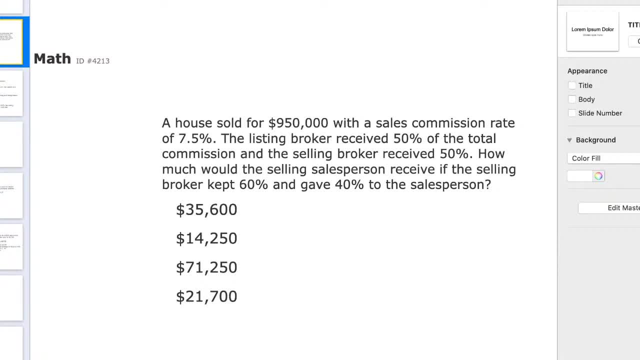 with the sales commission rate of seven and a half percent. the listing broker received fifty percent of the total commission and the selling broker received fifty percent. how much would the selling salesperson receive if the selling broker kept sixty percent and gave 40 to the salesperson? a 35 600, b 14 250, c 71 250 or d 21 700? what do you guys think? 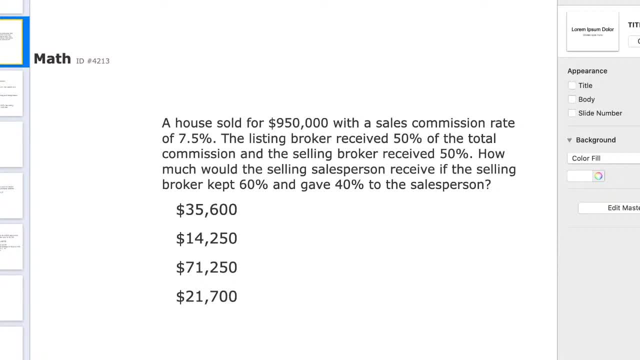 okay, or what's the first thing that pops out to you guys? what do you guys think? you guys don't just have to write the answer. you're more than welcome to share your thoughts of what you're seeing as you see this on the board. okay, and those of you guys who are watching this back, remember you could always pause it here and 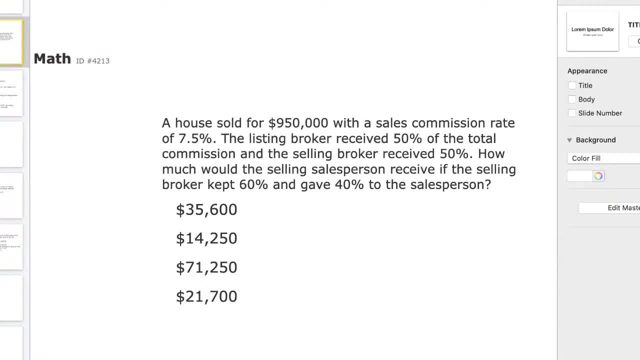 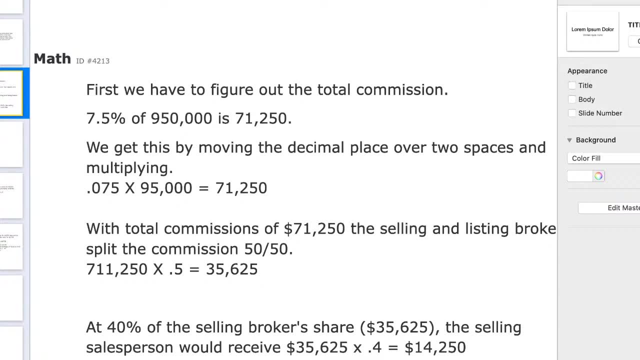 work out these problems. and all these problems are in the prep agent system as well, when you do math in our prep agent system. so how do we do this? okay, so first thing, we look at seven and a half percent of nine hundred fifty thousand. okay, so the house sold. 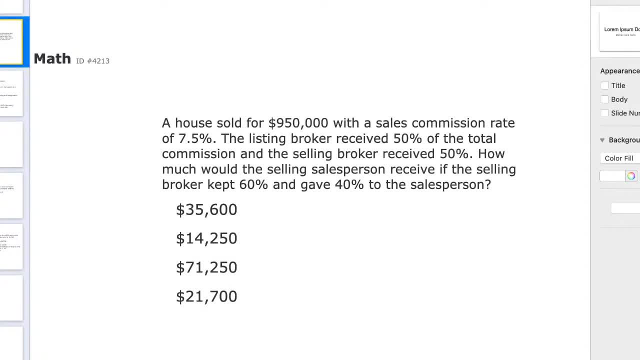 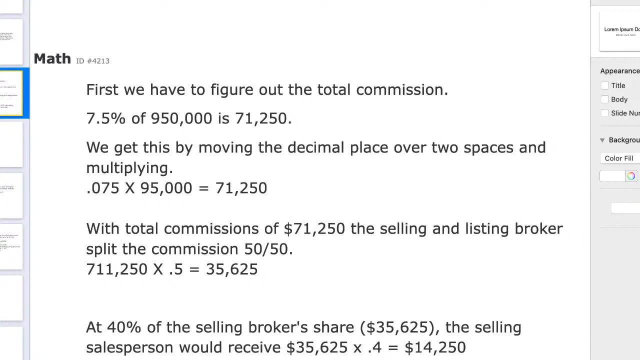 for nine hundred fifty thousand, with a commission of seven and a half percent. by the way, that'd be a huge commission. they're not normally that big, that'd be crazy. but whatever, normally it's like a lot less than that. but they give you these big numbers to give you encouragement, which i guess i 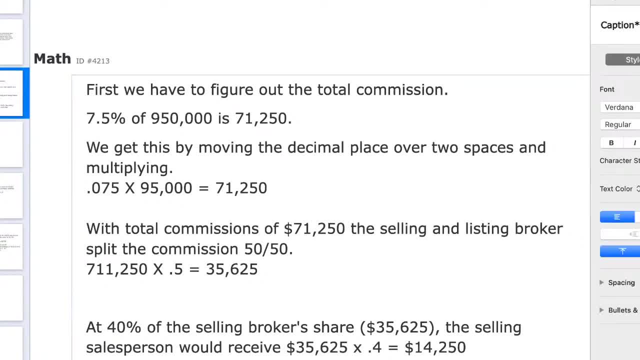 should too. okay. so that's seventy one thousand two hundred fifty. remember, when we multiply we move the decimal place over two spots. so it's point zero, seven five times ninety five thousand. joseph said they are in california. the price the house may be, but the commission is not. 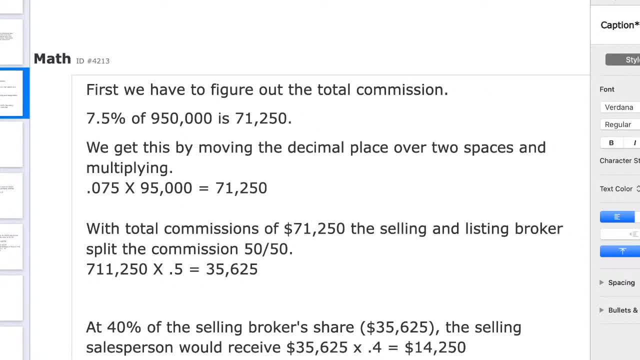 the percentage. um, okay, so point oh, seven five times ninety five thousand is seventy one thousand two hundred fifty everybody with me so far, right, got it. so that's the commission for everybody. uh, does everybody understands who the selling broker is? this confuses a lot of people. 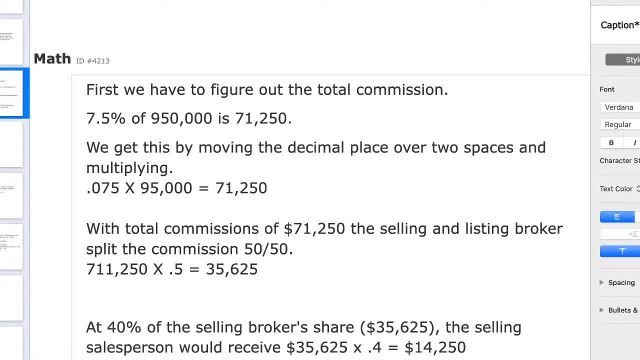 not just on math but also in general when you see questions on your exam. the selling brokers, the one who brings the buyer. i know they say buyer broker and selling broker, but if you actually look at a listing for a broker in any company there's a commander, then there's a supplier now, so that's the one who's paying as far as it作لا 이� packets. so a agency is not helping an agency abroad which, if that can help offense brokers. instead, Misses taped their American and develop another business union group. well, because olivares r-ueloo, i appreciatepack team. I know they said buyer broker and selling broker, but if you actually look at a listing, 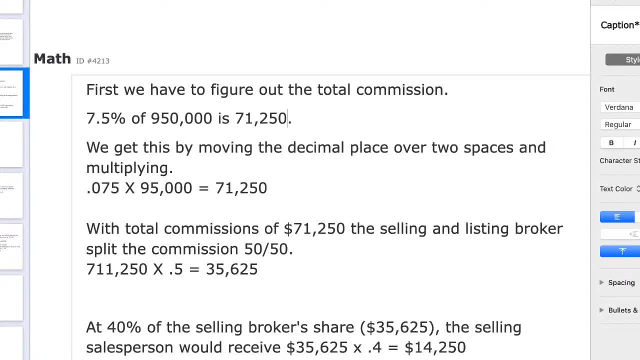 listing contract. okay, it'll actually say selling broker and listing broker. the selling broker brings the buyer, the listing broker is the one who represents the seller. everybody got that. people get confused with that. okay, all right, so it's 50: 50, so they both split 35 625. 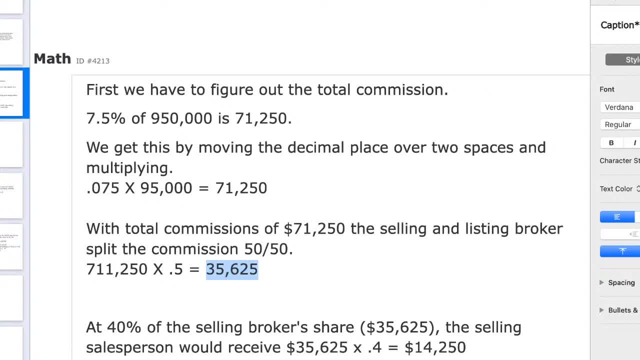 the 40 of the selling brokers share 35 625. that's a share. the salesperson will receive 35 625, that's times 0.4. remember, you have the brokers and they may not actually be doing the deal. okay, the agent is the one doing the deal, but they work under that broker, the broker's name, that. 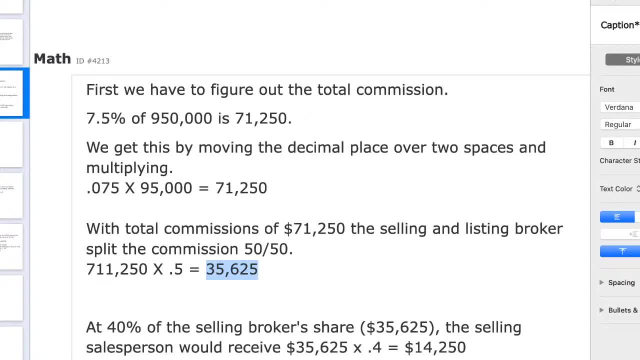 goes on the dotted line, okay, and then the agent has their split with the broker, right, and this is their split, okay, everybody got it. so hopefully you see the reason why you want to be able to do commission problems, not only because, well, frankly, i bet you guys, all of you, have done commission problems. 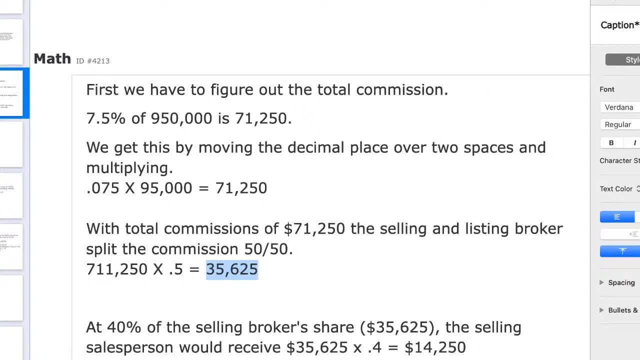 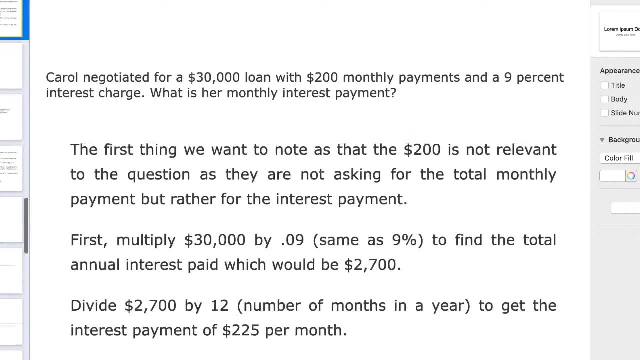 already. that's why you're here, that's why you're doing this exam. you had a friend sell a house. you did the commission. you're like what i need to get my real estate license. i'm all over that, right, guys? okay, let's do another one. 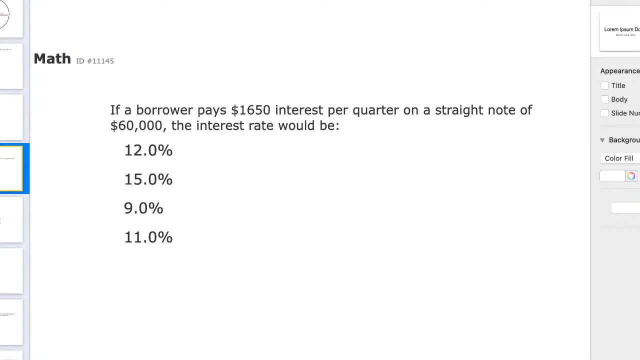 all right. if a borrower pays 1650 in interest per quarter, on a straight note of sixty thousand dollars, the interest rate would be a 12 percent, b, 15, b, 15, c, 9 and d 11. and bruce says 0.075 is the same percent as 7.5. yeah, it's a great point, bruce. 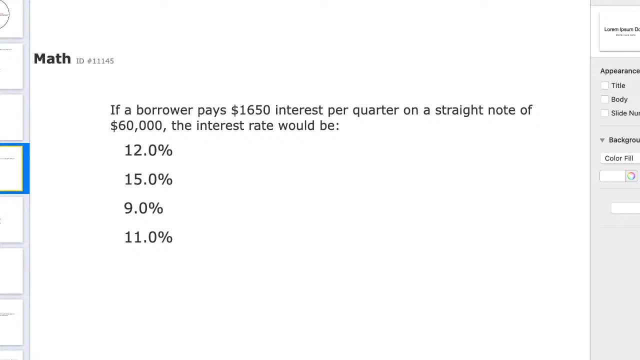 thank you for writing that. just remember, when you see the percent to move the decimal place over two spaces. so 7.5, as bruce wrote, is point zero, seven, seven, seven percent, five. okay, so if a borrower pays 1650 interest per quarter, straight note of sixty thousand dollars. 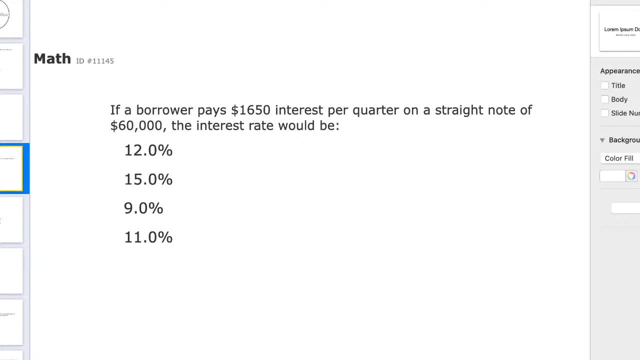 the interest rate would be okay. first thing you guys should notice here is: what? don't give me the answer. i don't want your guys answers. i want to know what's the first thing that should pop out to you here. what do you guys think what's the first thing that should pop out? what's a word? 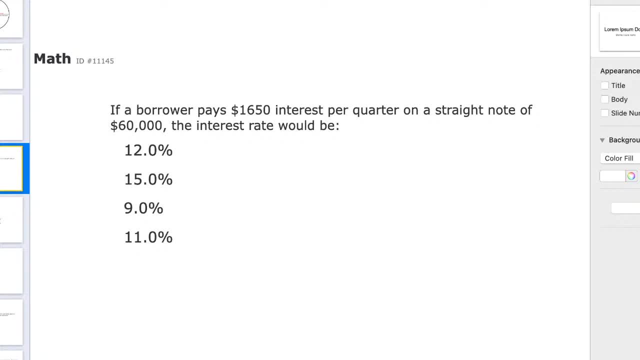 here. that would make you go: oh quarter. excellent job, joseph quarter. if you guys heard my webinar two weeks ago on math and i'll repeat it is: you must always try to default to annual figures unless they designate otherwise. everybody got that. everybody write that down: default to annual. 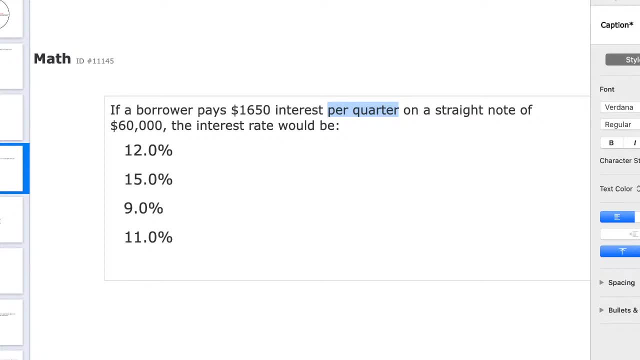 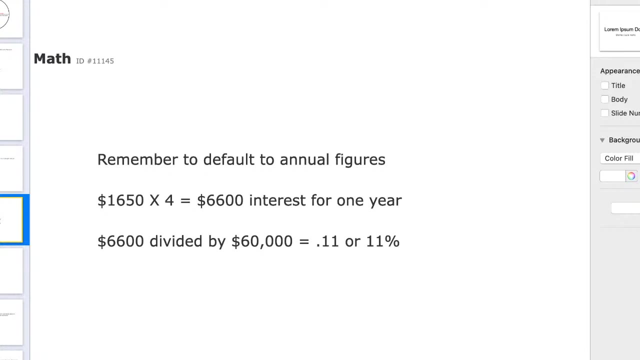 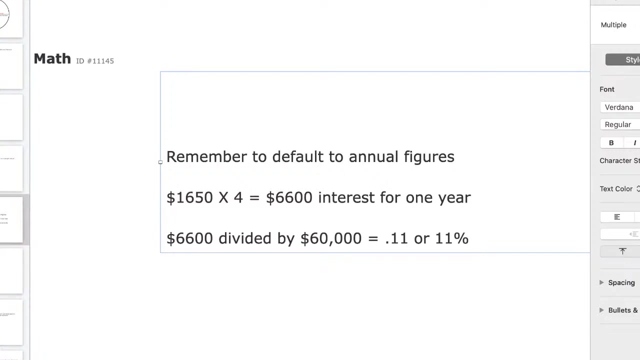 figures, default to annual figures. okay, everybody got that. so you always want to default to annual figures. so you see quarter and what must we do? so we default to annual figures, like i said before. it says right there: and you take the 1650 times four, which equals 6600 interest for one year. 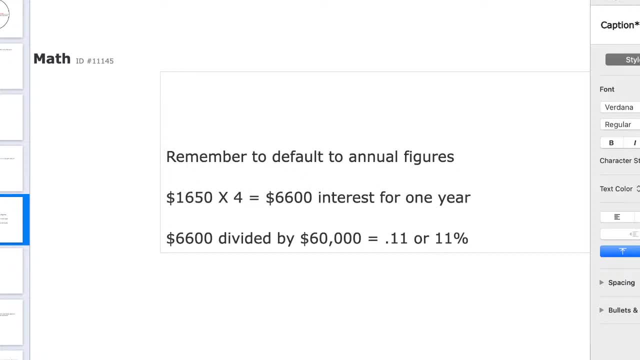 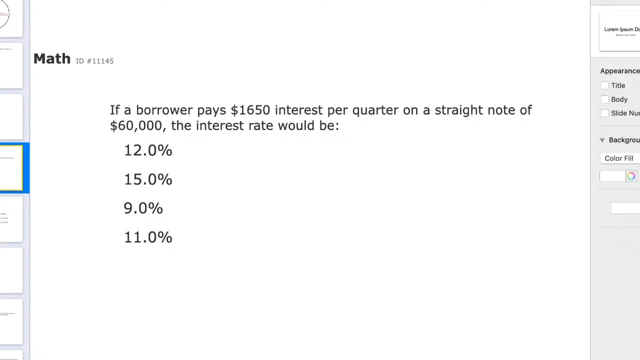 and then to figure out percentage, you take that number, you divide it and you get 11 percent. point 11 equals 11 percent. when they say: what percentage is 60 000 of that number? we just multiplied the 6600, you get 11 percent. okay, 6600 is 11 percent of 60. 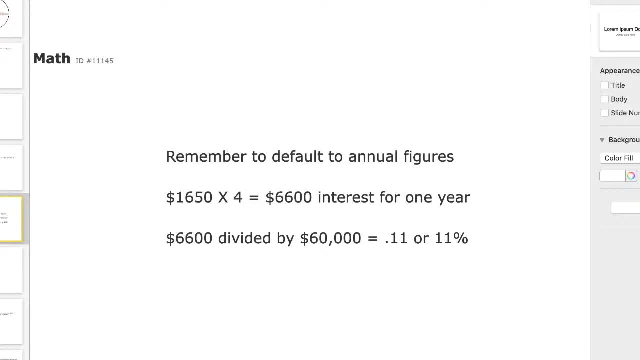 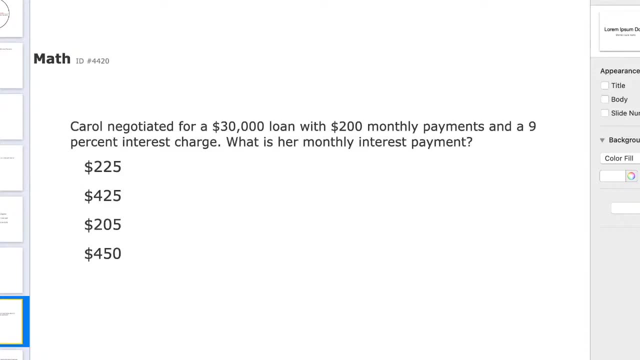 percent. so if you get that number, do we know or not we're going to? um, we could do a whole lot of different things with that. so y'all just have to read this one, because we're gonna do the math. you're gonna get a. yeah, if i move down here and i'm gonna do something, just like that. and the math. 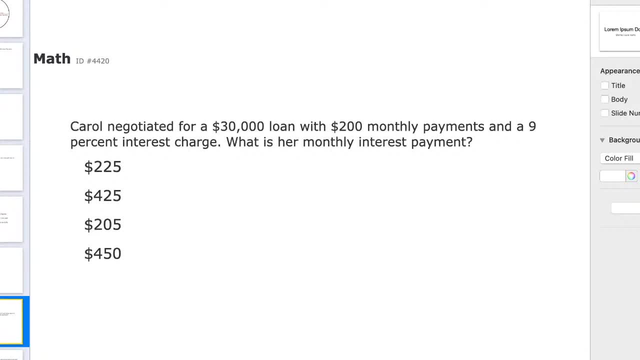 goes in like this: see how it's moving. if you're wrong, you're gonna find what was wrong and you're gonna make a new one, and then you're gonna find something that's wrong, and then you're gonna do something that's wrong and you're gonna try that and you're gonna make a new one, and then you're gonna. 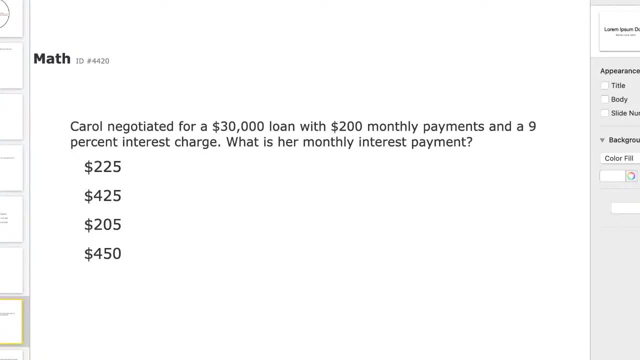 just build it and then you're gonna repeat it like you're going to a lot more and then you're gonna problems all day. okay, Carol negotiated- I totally hear my accent when I say the word Carol. Carol negotiated for a $30,000 loan with $200 monthly payment. 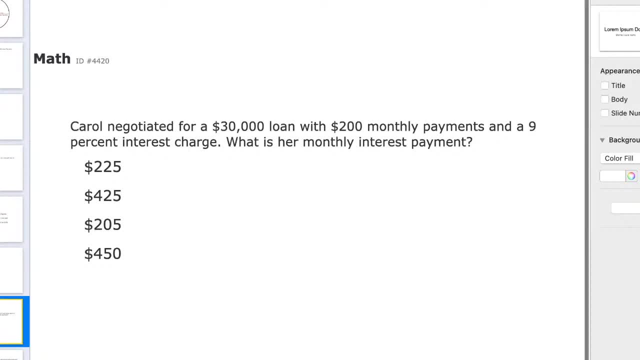 and a 9% interest charge. what is her monthly interest payment? a, 225, B, 425, C 205 or D 450? first thing that should pop out to you here is: what? what do you guys think we read this question? what should pop out to us here? okay, what? 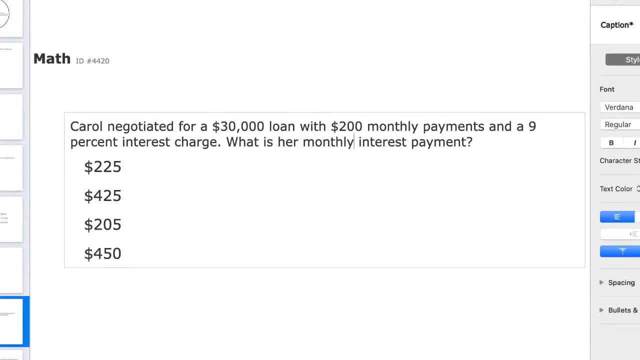 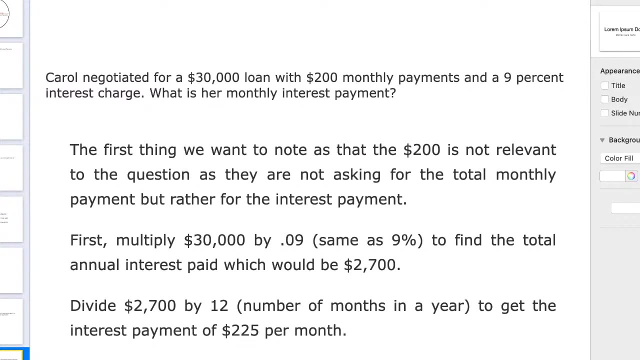 should pop out to us here is: they're asking about the interest, interest payment- and they're saying $200 monthly payments. that's not the relevant factor, okay, okay. so we look at this question. Carol negotiated for $300,000 loan with a $200 payments and a 9% interest charge. so they're not saying that that that interest charge is. 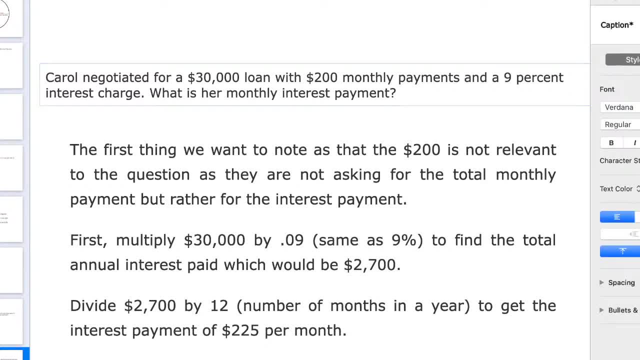 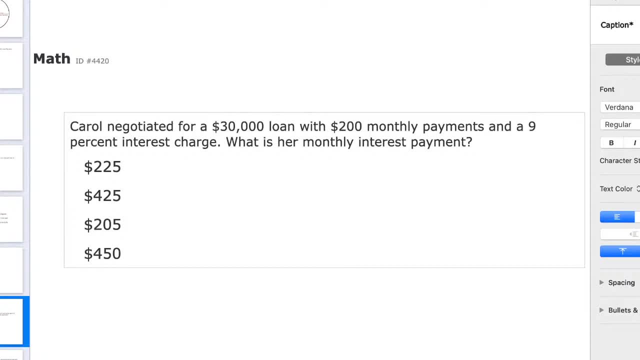 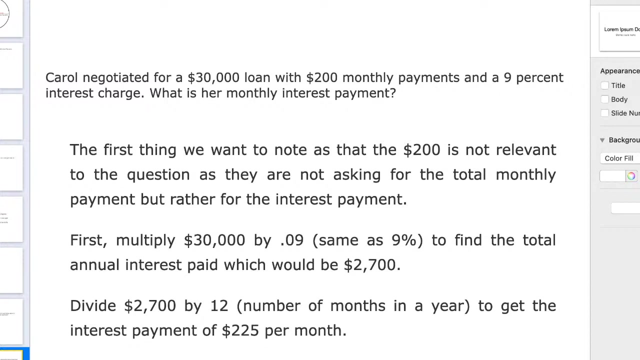 part of the 200. everybody see that says: and a 9% interest charge. gotta read that carefully. it's tricky, right, everybody right tricky. it says: and a 9% interest charge. okay, everybody got that. so first thing we note is that the 200 is not relevant to. 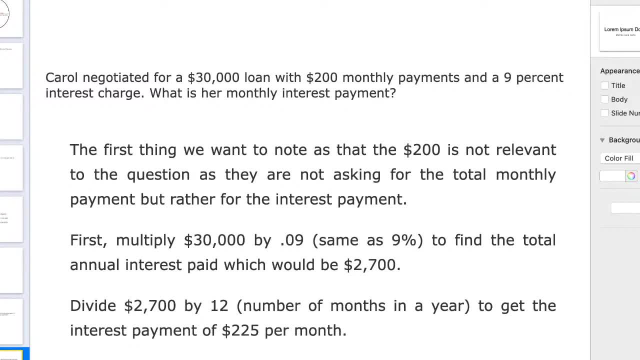 a question is: they are not asking for the total payment, but rather for the interest payment. who missed that? I know I missed that the first time. I saw that. okay, but you gotta see that. once you realize that, then the rest is is a cakewalk, but you. 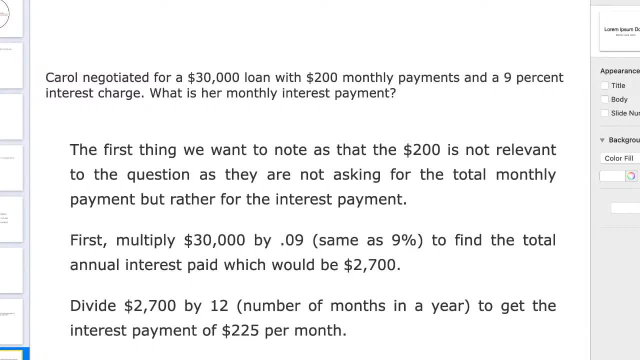 gotta spot that because i know when i saw the two hundred dollars i was like, oh, i'm so scared. okay, so first multiply the 30 000 times 0.09, as that's nine percent, to find the total annual interest payment, which would be 2700. now, as many, you point out correctly what also stuck out to you: 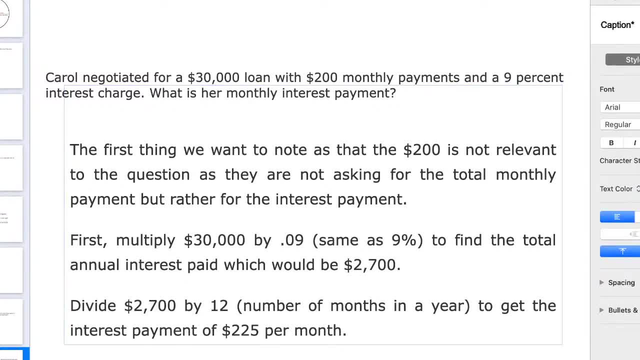 is they're asking about monthly, the monthly interest payment monthly. so what does that mean we need to do? we need to divide it by 12 and we get the answer of 225 dollars a month. all right, hopefully a lot of the stuff is coming clear and i can see why i get frustrated. if you're. constantly trying to work the 200 dollars a month and you're constantly trying to work the 200 dollars a month. all right, hopefully a lot of the stuff is coming clear and i can see why i get frustrated if you're constantly trying to work the 200 dollars a month and you get the answer of 225 dollars a month. 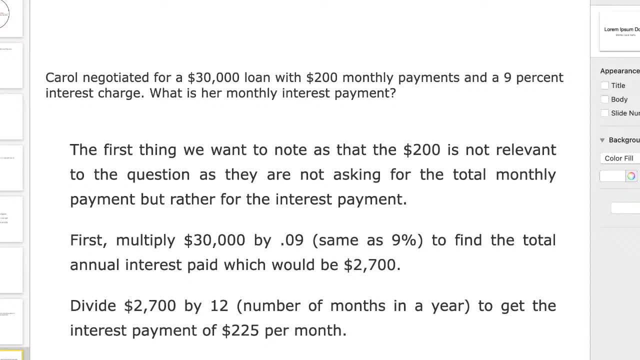 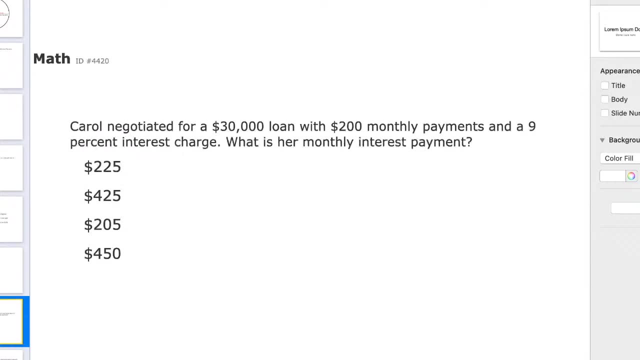 all right. oh, vita, terry brought a great point. if you circle the 425, then the state department is saying: got. ya, you didn't read it correctly. um, because you guys could easily say, oh, that plus the 200 and i get 425, all right, so you guys got to be careful. so, because they're asking about 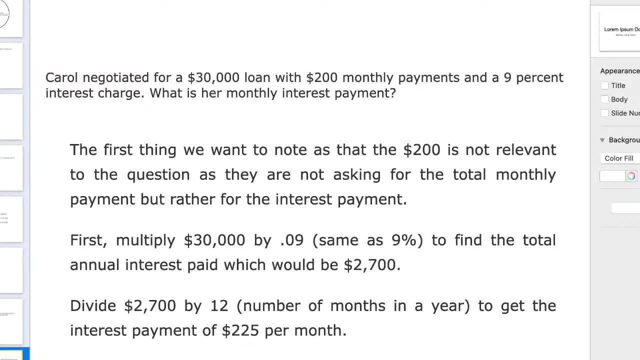 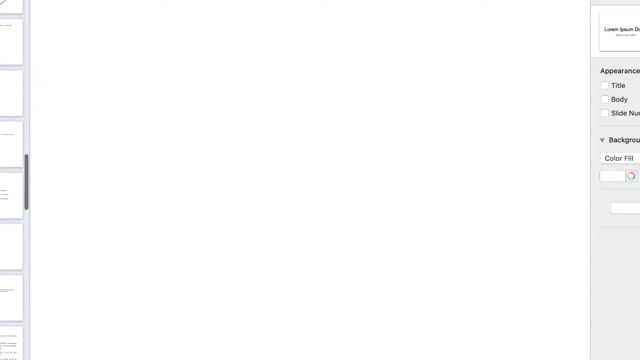 monthly. we default to the annual figures. you need to divide that by 12 and you get 225 per month. all right, that's right, Dante. sometimes to give you numbers you don't need totally annoying. okay, a homeowner sold his house for $230,000. the selling 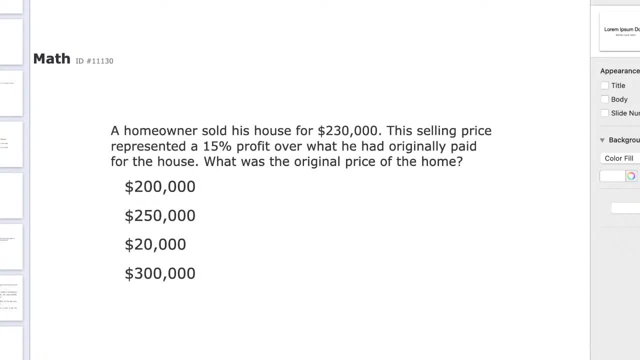 price represented a 15% profit over what he originally paid for the house. what was the original price of the whole? a $200, B $250- see on $200, I'm sorry, $200,000. be $250,000, see $20,000. or D $300,000. what do you guys think? 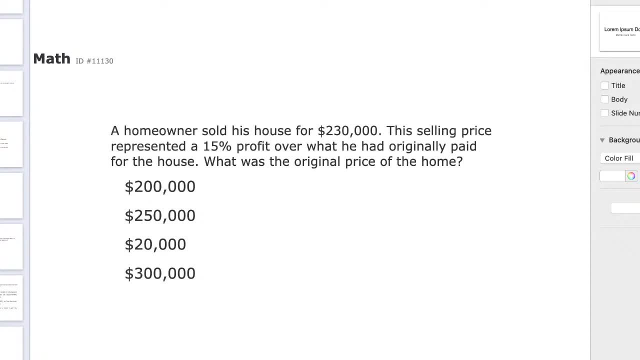 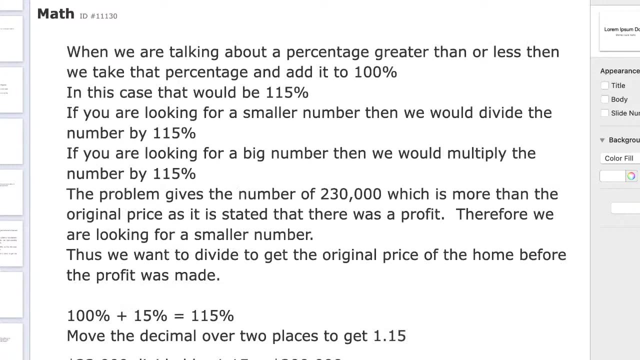 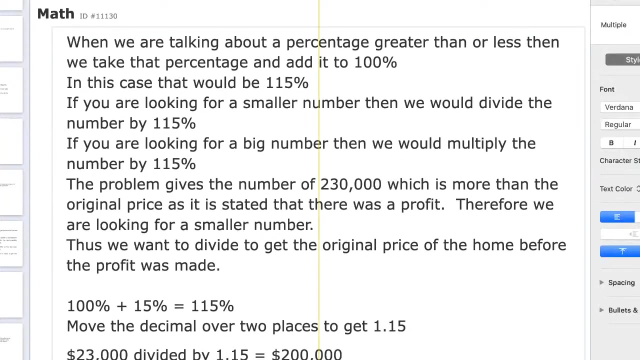 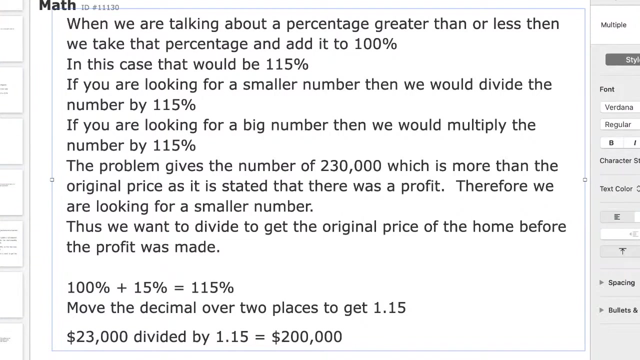 all right, whoo, I wrote a long explanation here for you guys cuz I love you. okay, see if I can move this up here for a little for you. there we all see what I wrote. maybe I should have done that on two slides, oh well, okay, we're talking about. percentage is greater than or less than we take the. 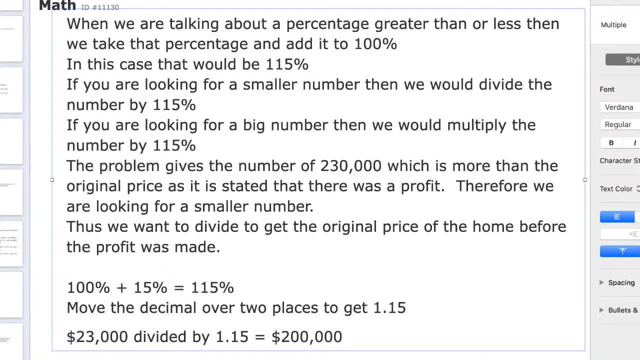 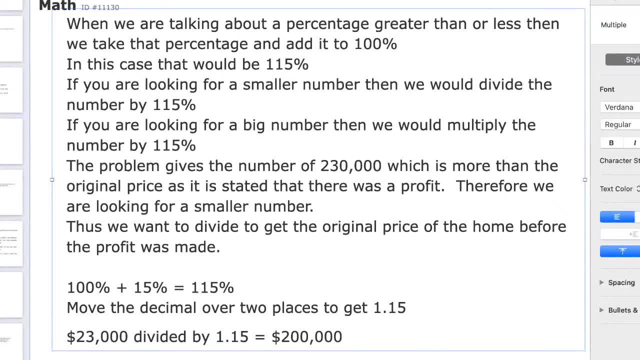 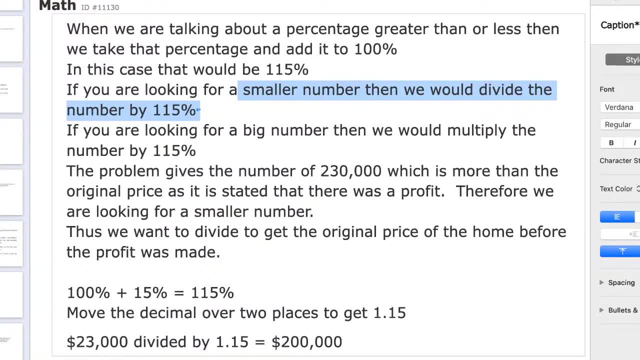 percent. okay. so that's important there. if you're looking for a bigger number, then you would multiply it by the hundred fifteen percent. the problem gives us the number of 230,000, which is more than the original price, okay. so therefore you know we're looking for a smaller number they're asking us for 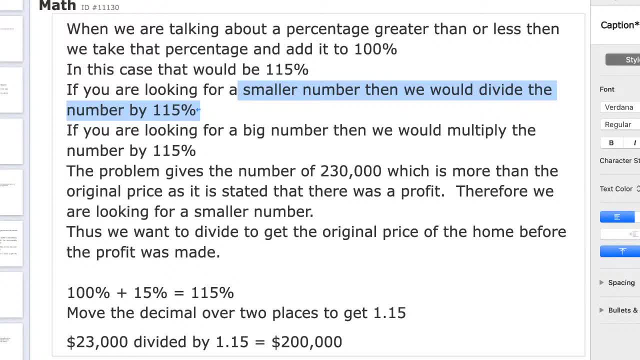 the original price, and we know that the original price is less than. excuse me, the price we're looking for is less than the original price. all right, okay, the problem gives us number 230,000, which is more than the original price. as they said, there was a profit. alia says: why 115? well, the reason is because the 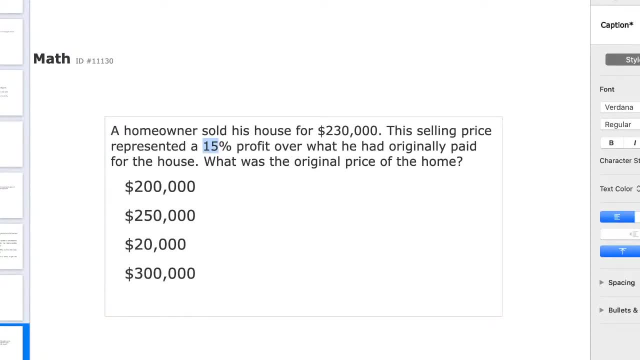 the problem gives us number 230,000, which is more than the original price. as they said, there was a profit alia says why 115? well, the reason is because the profit alia says why 115. well, the reason is because the profit alia says why 115. well, the reason is because the 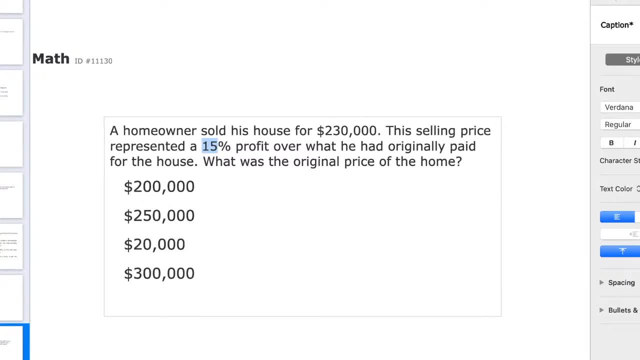 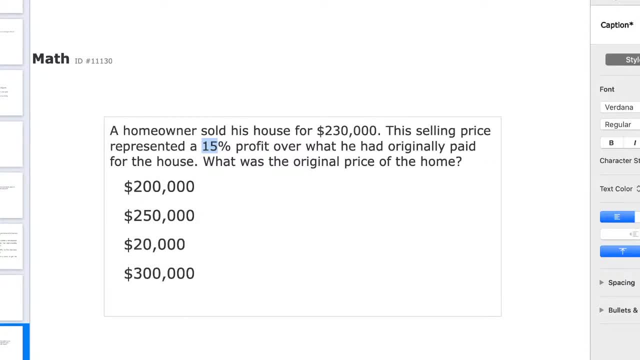 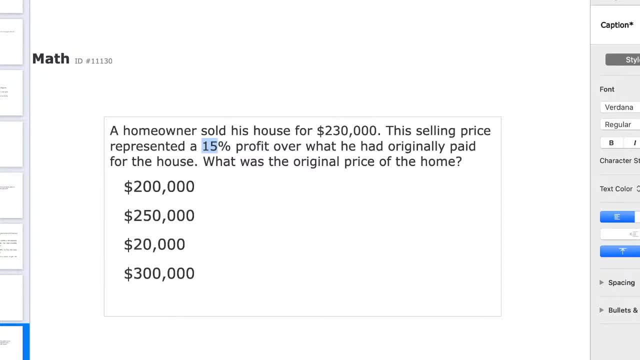 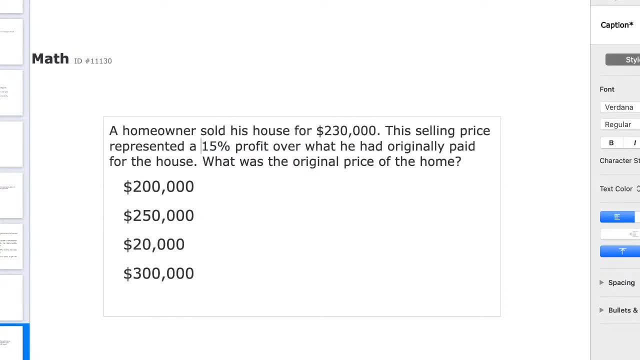 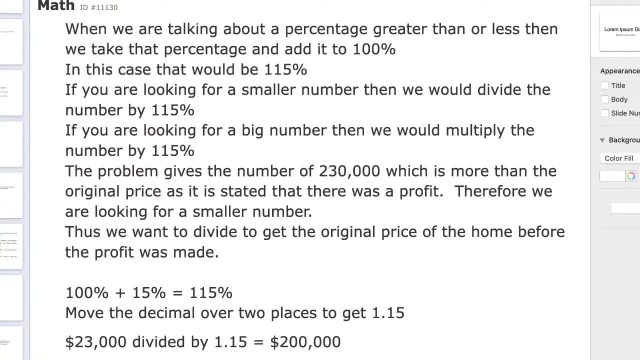 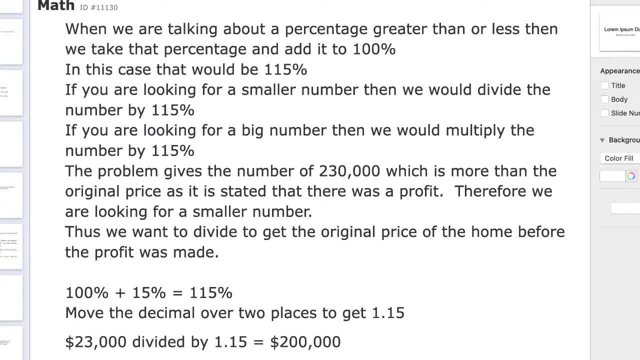 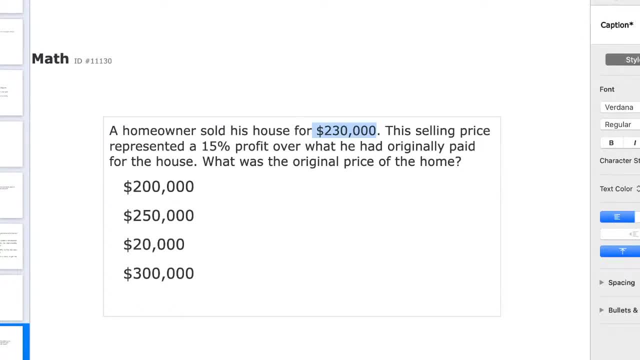 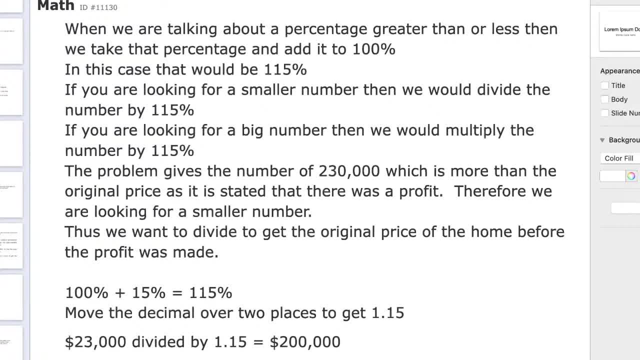 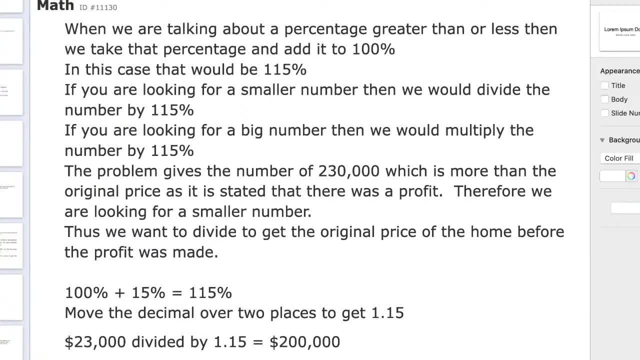 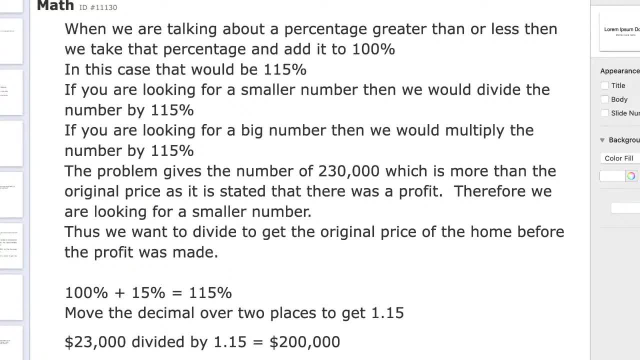 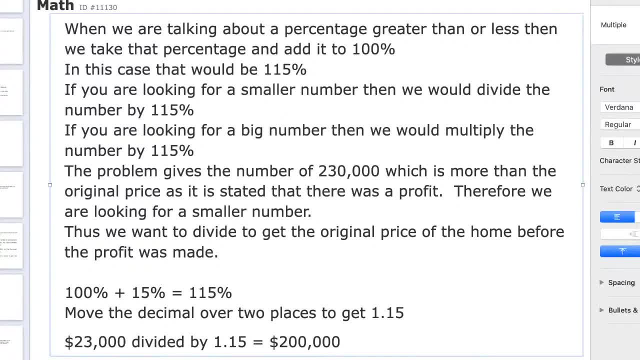 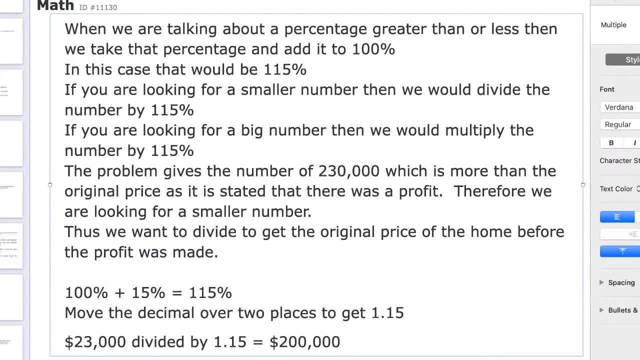 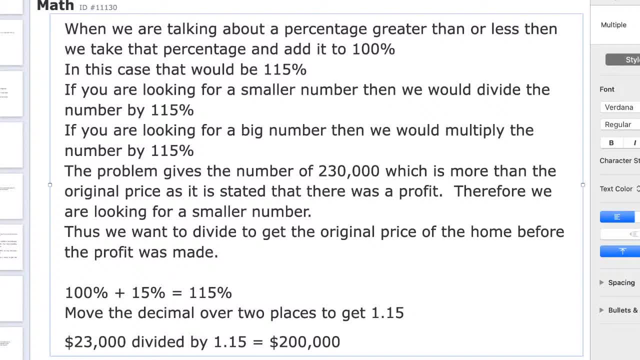 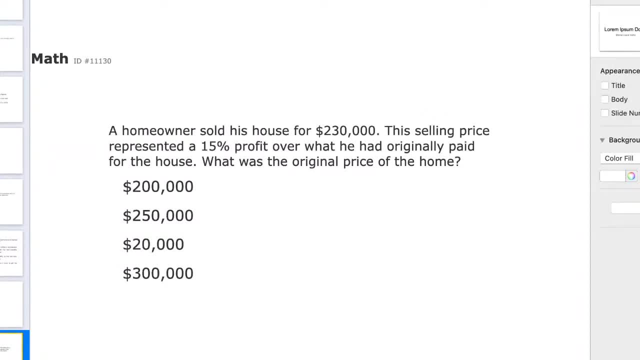 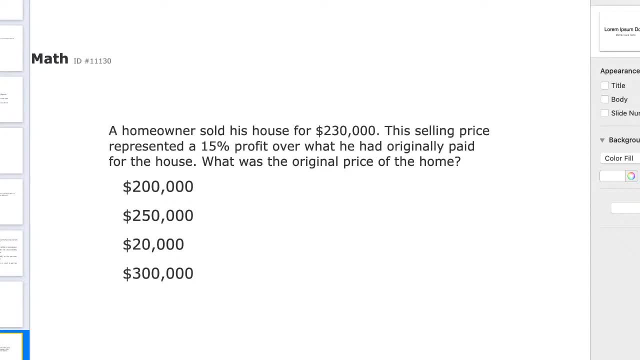 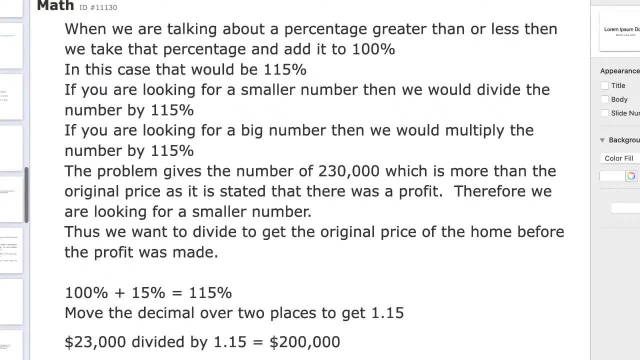 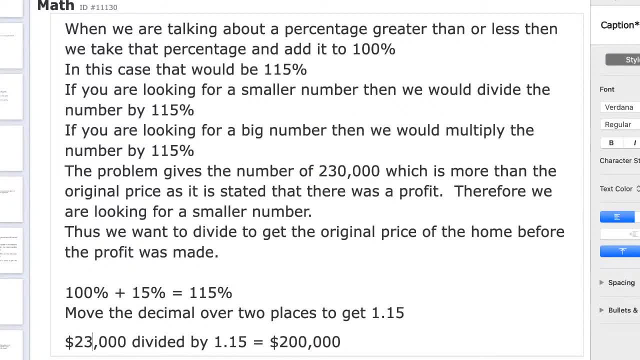 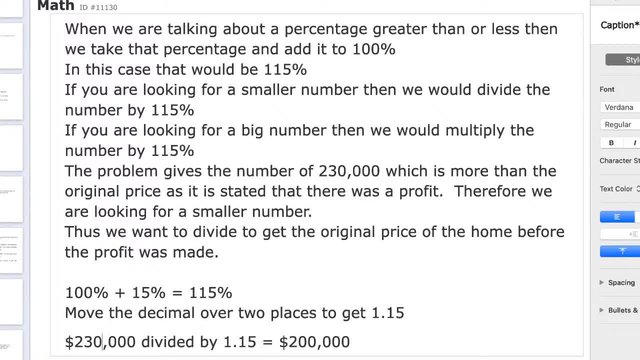 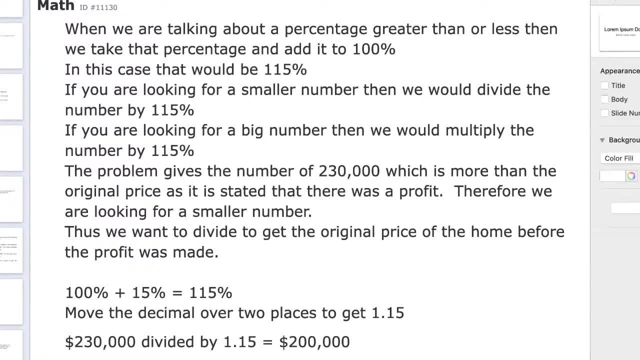 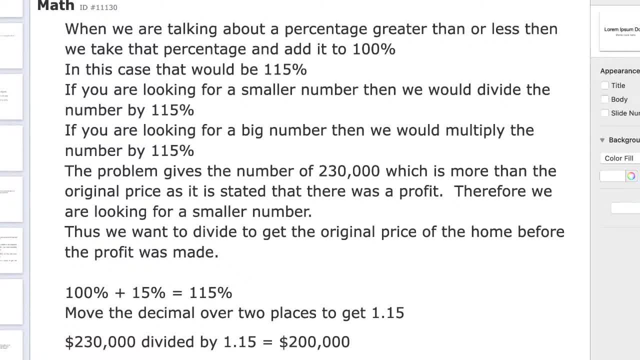 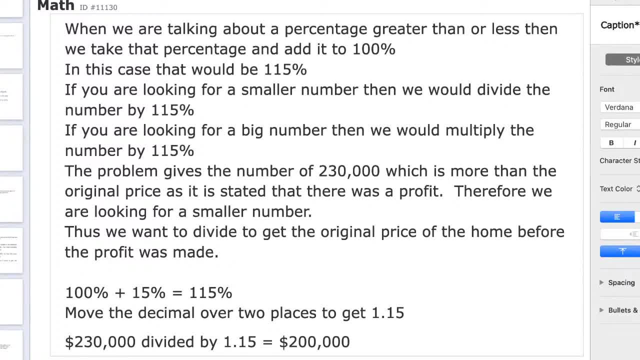 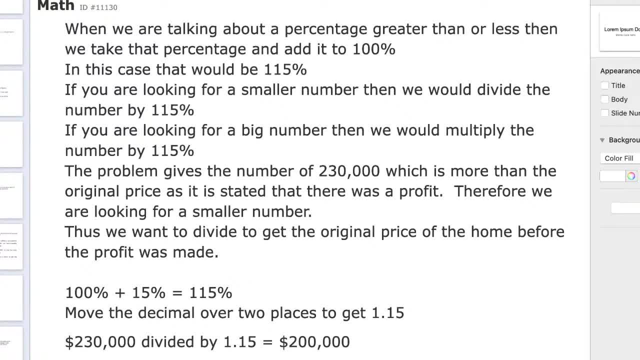 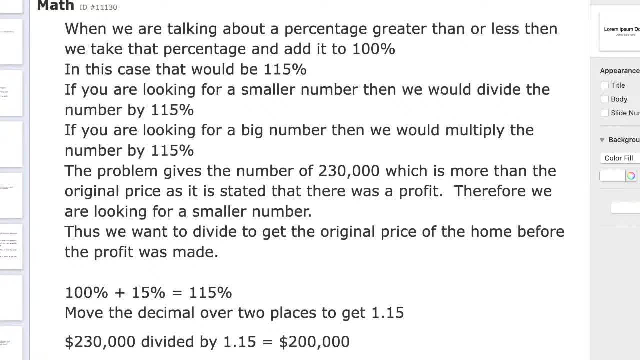 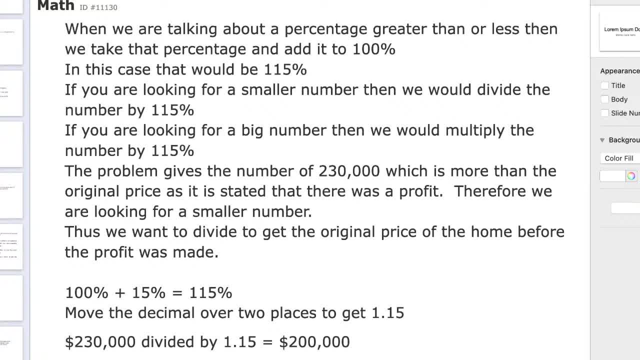 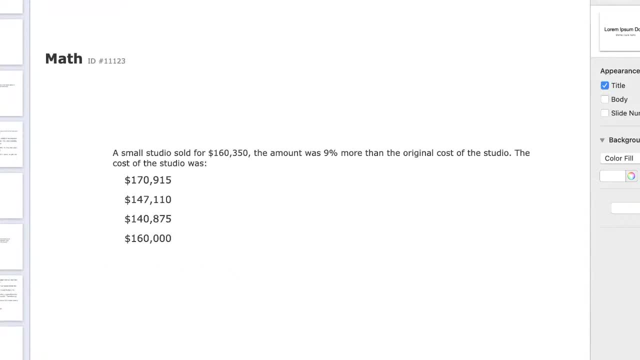 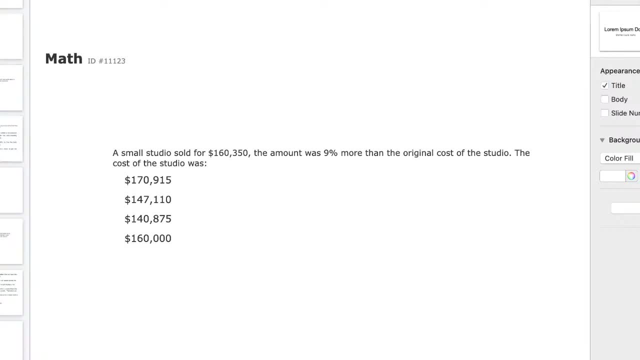 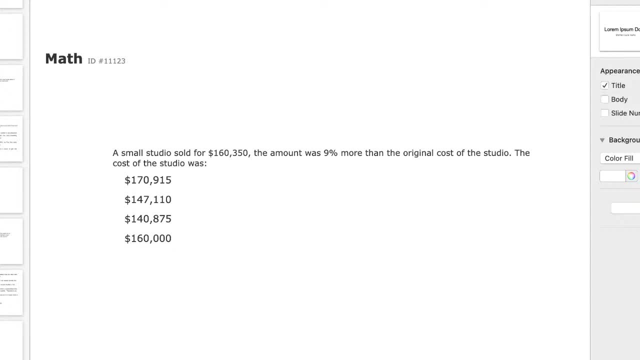 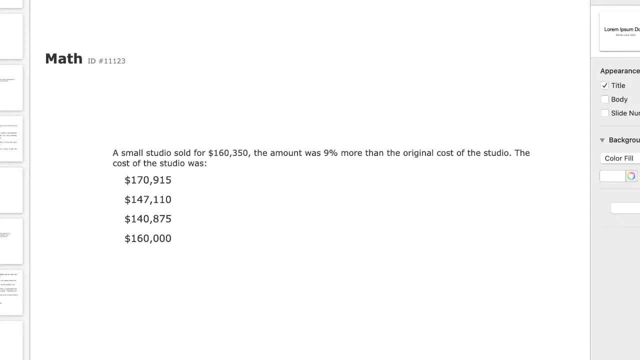 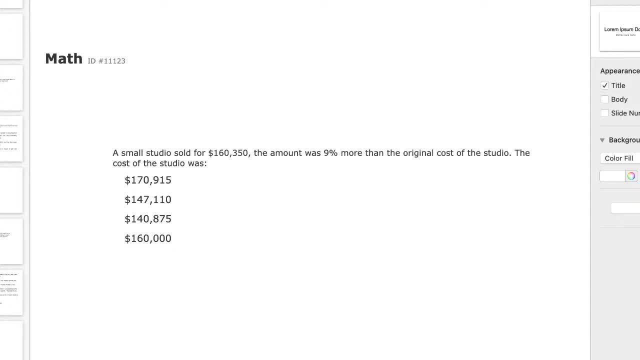 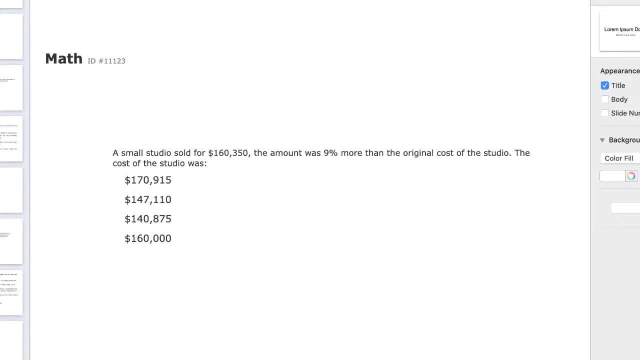 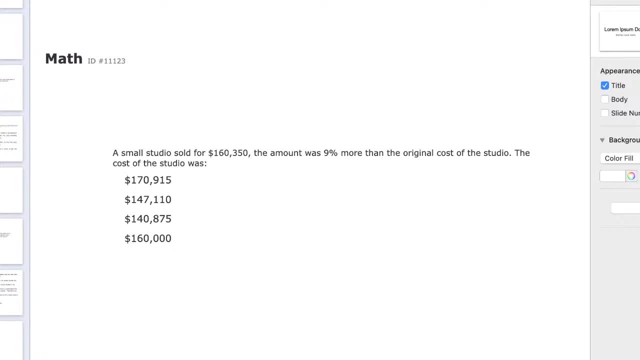 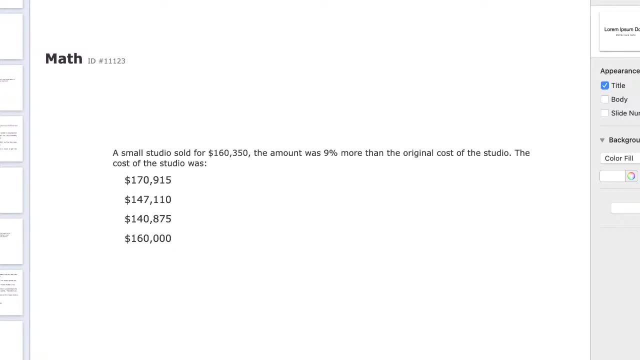 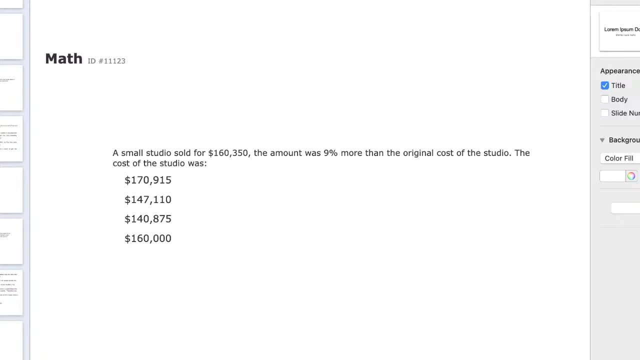 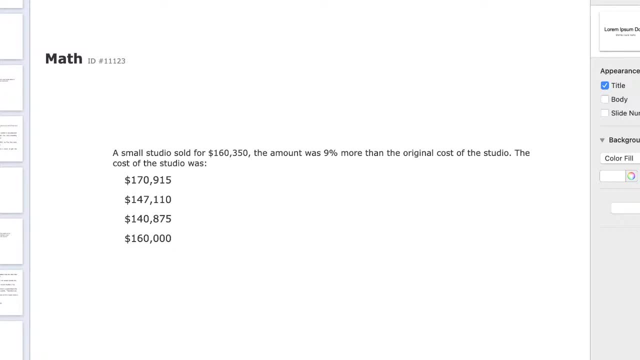 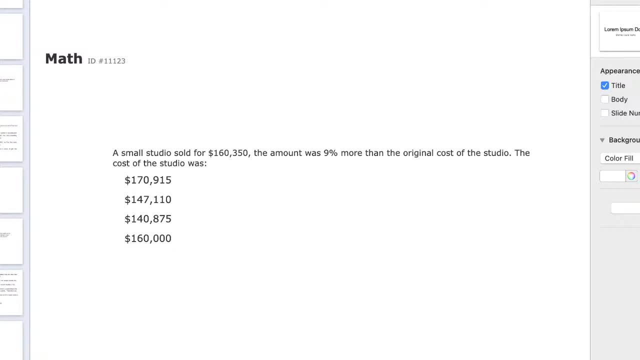 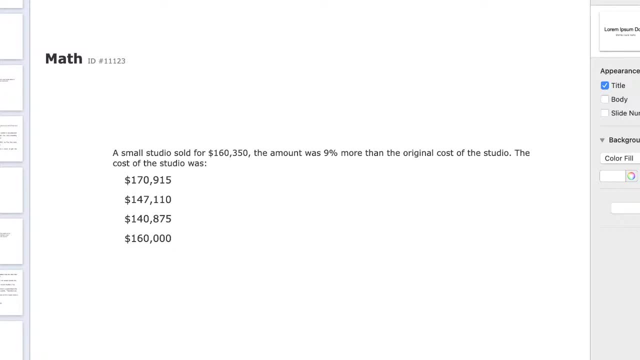 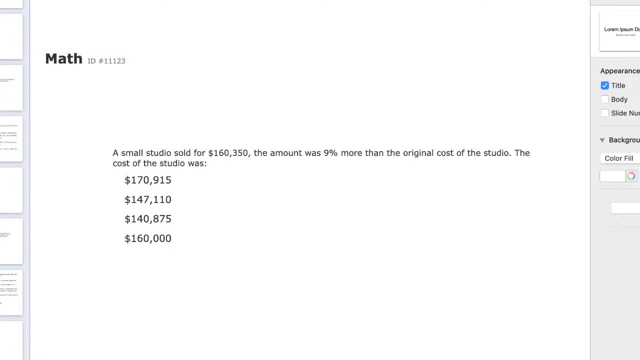 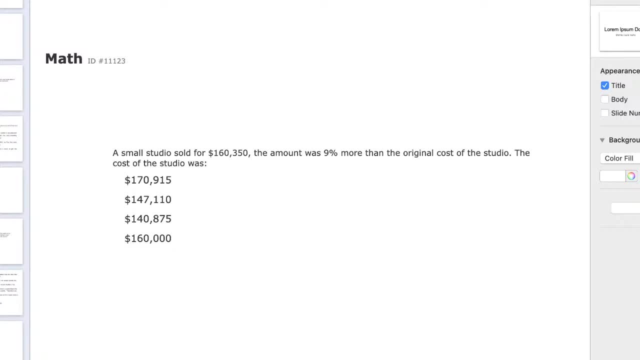 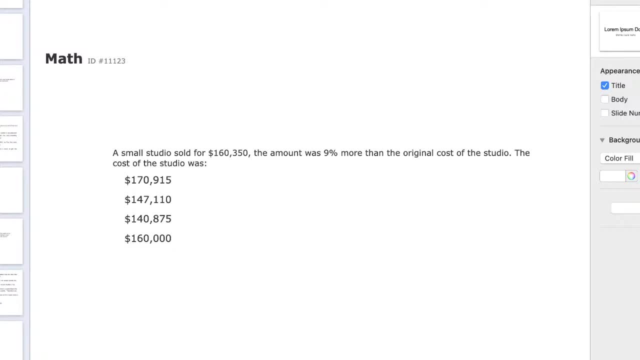 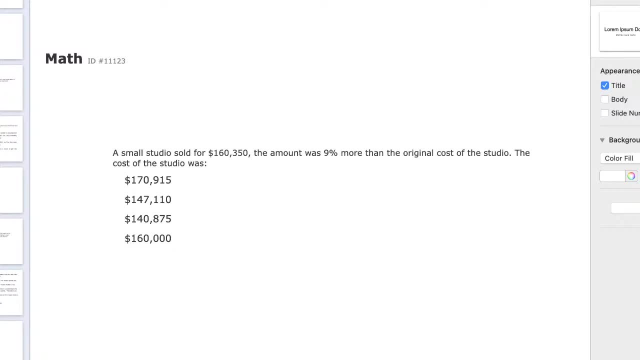 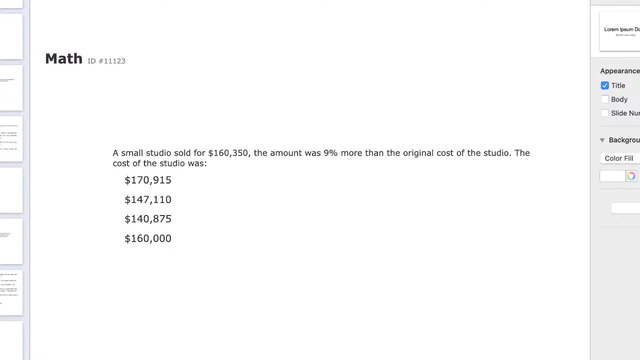 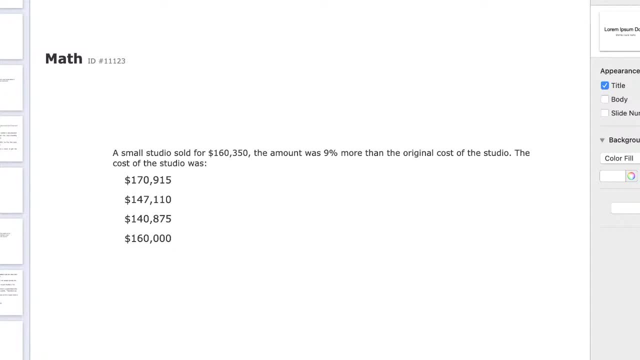 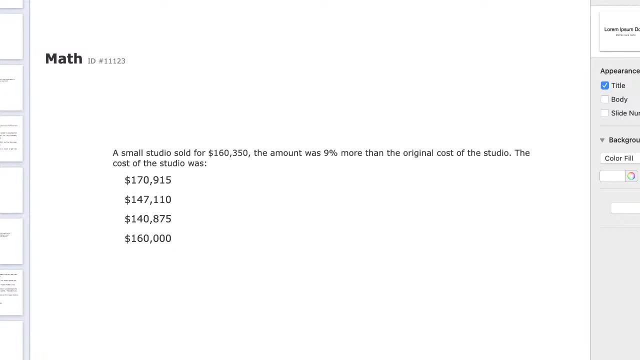 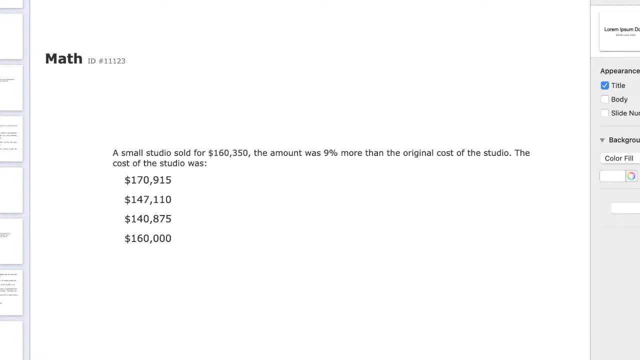 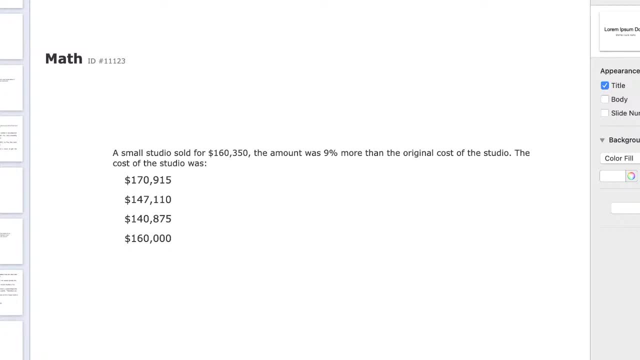 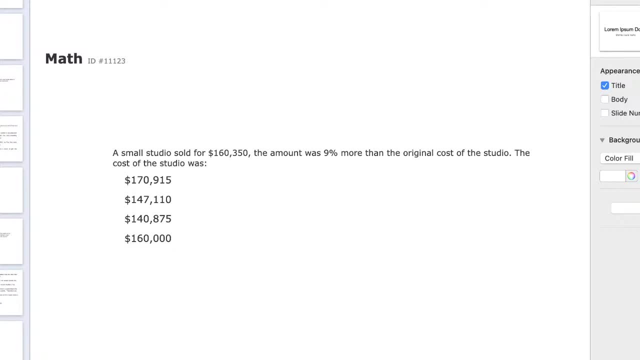 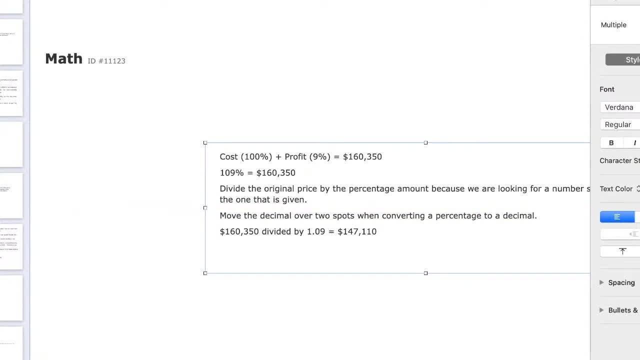 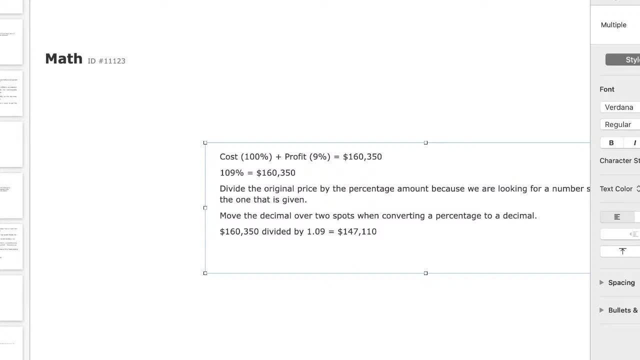 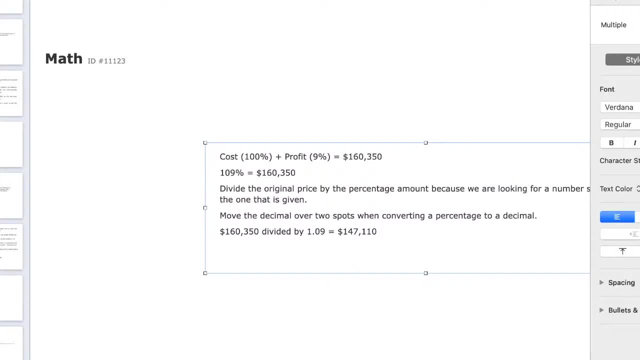 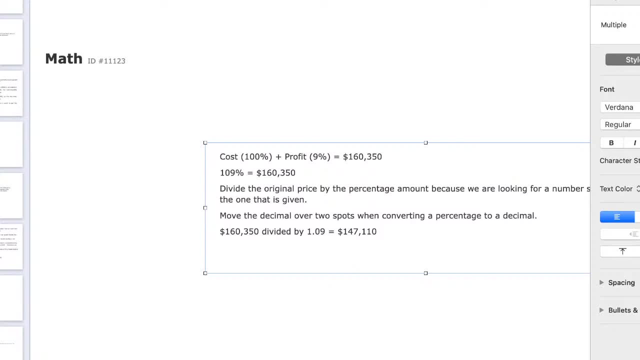 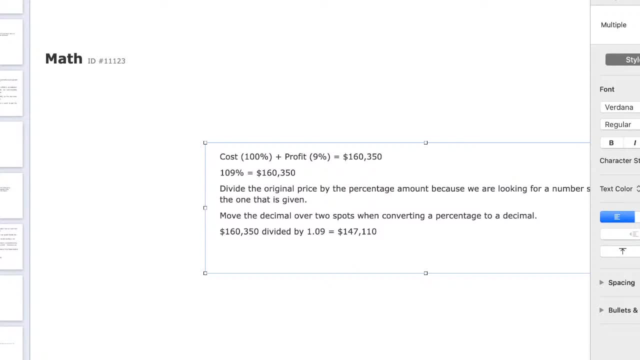 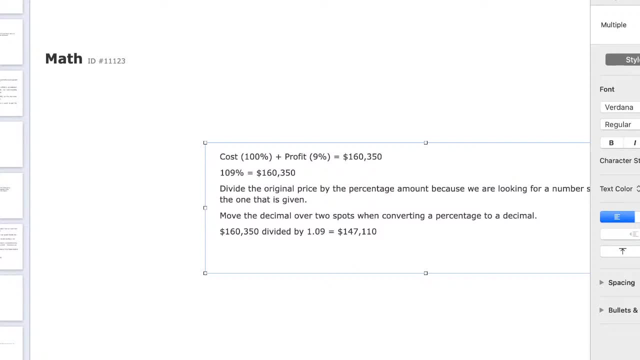 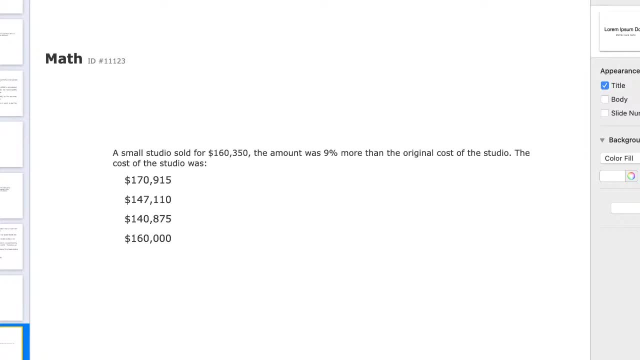 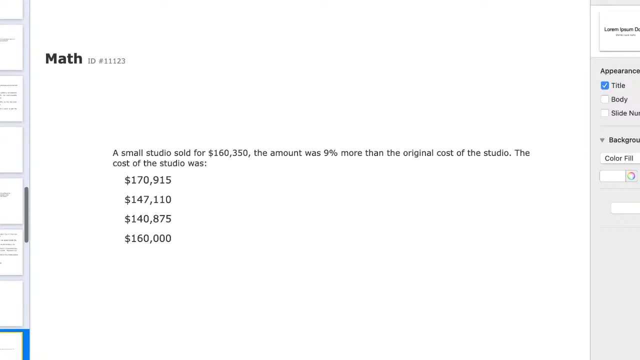 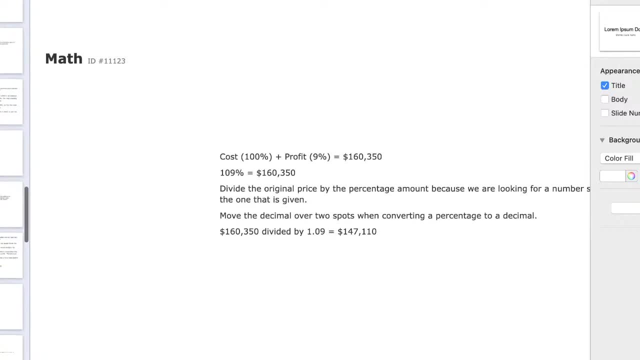 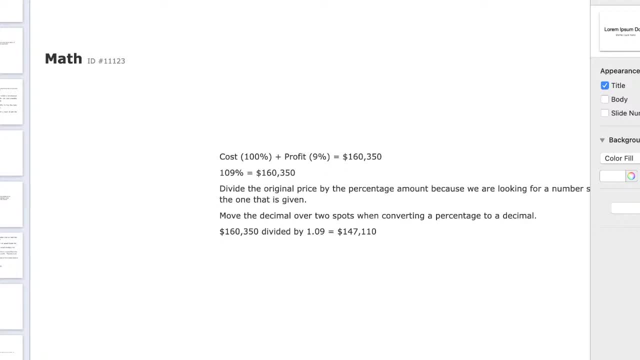 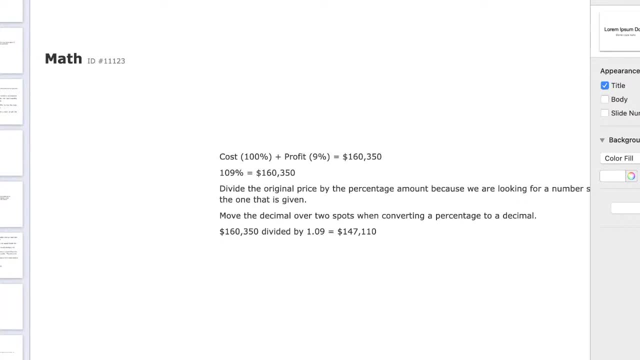 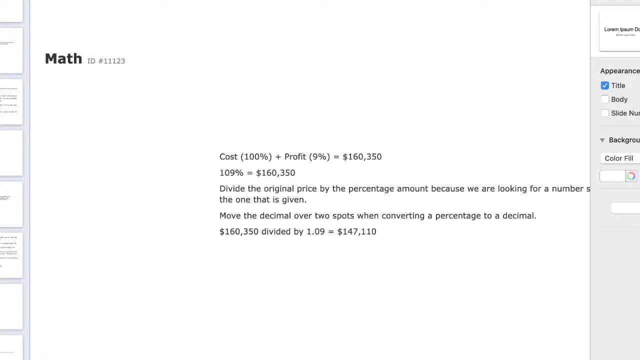 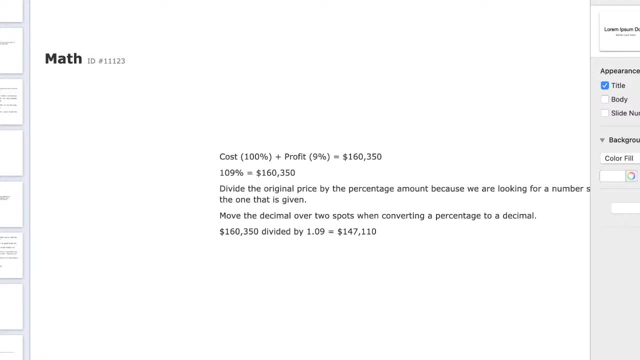 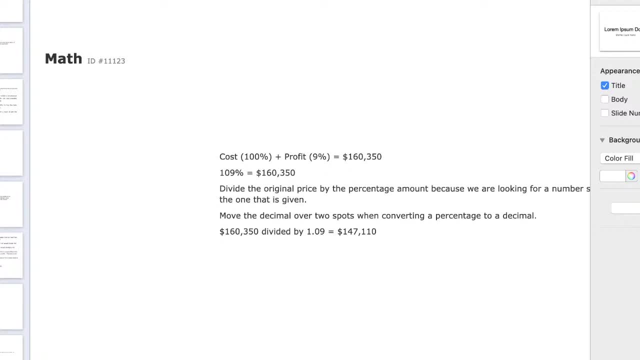 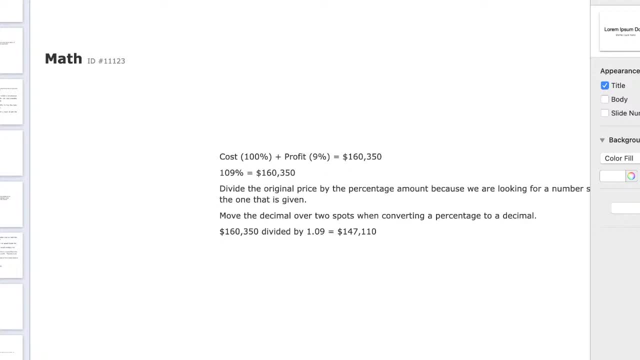 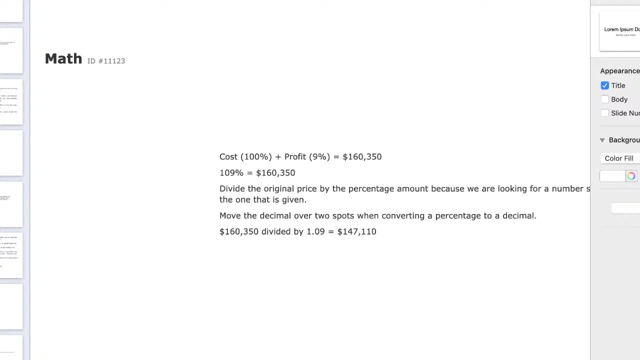 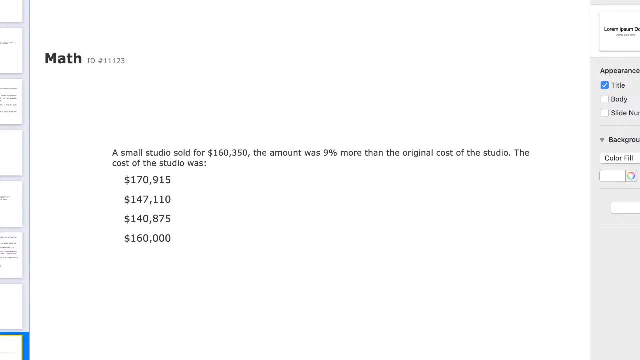 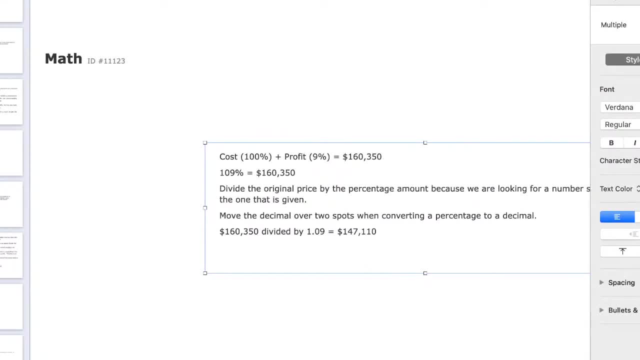 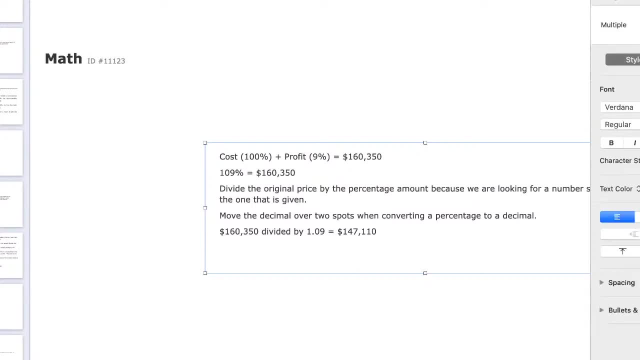 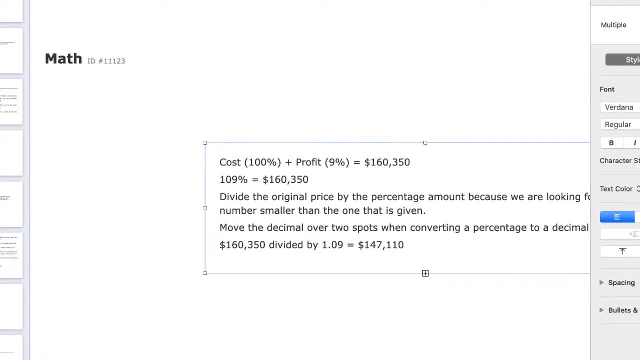 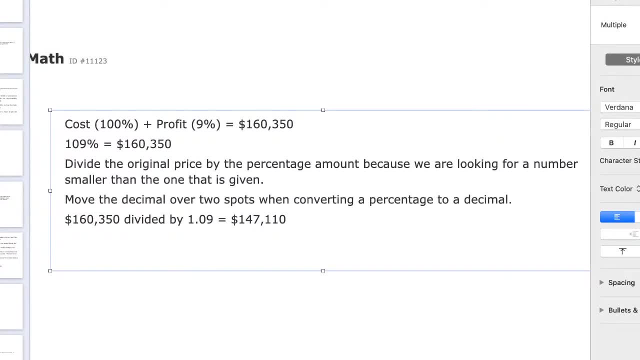 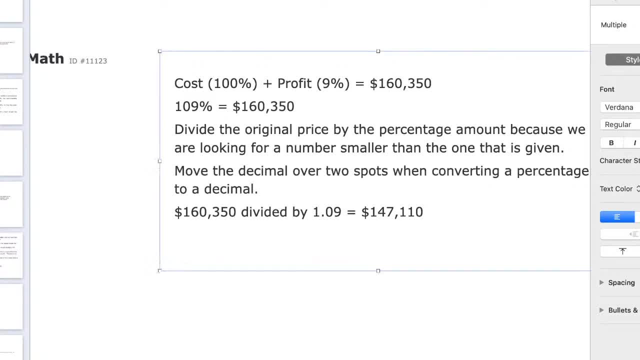 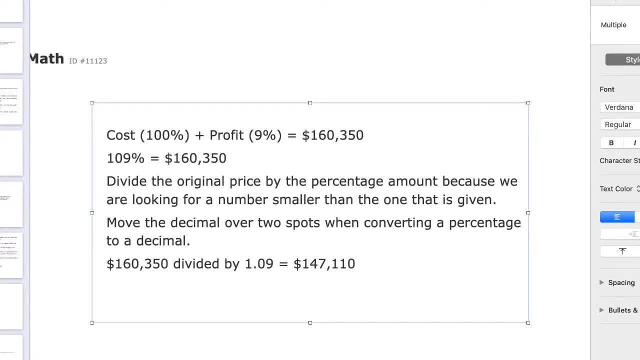 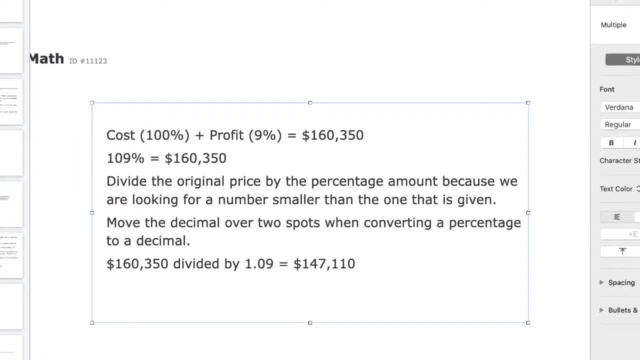 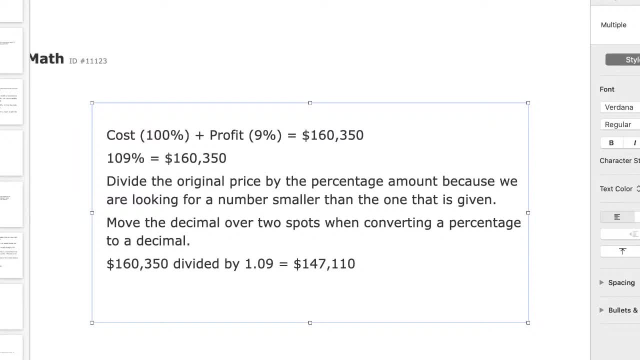 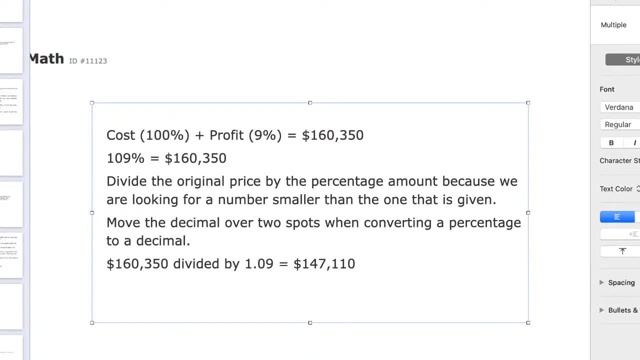 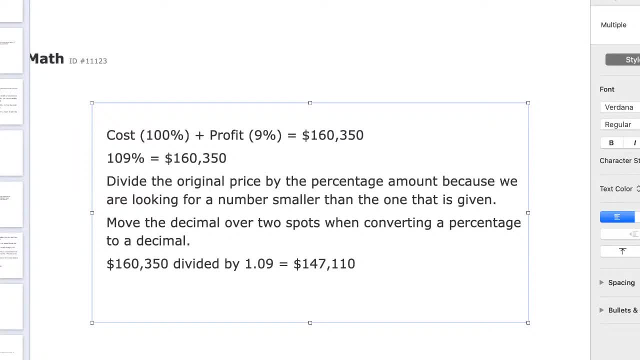 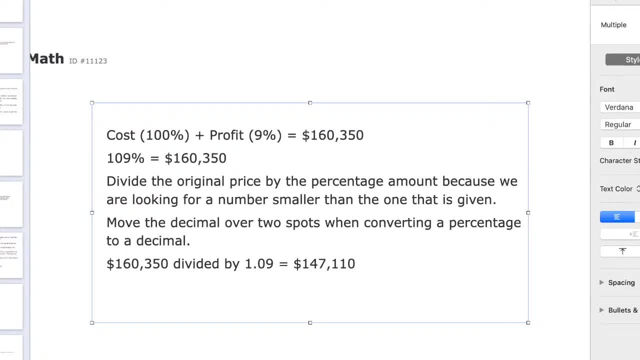 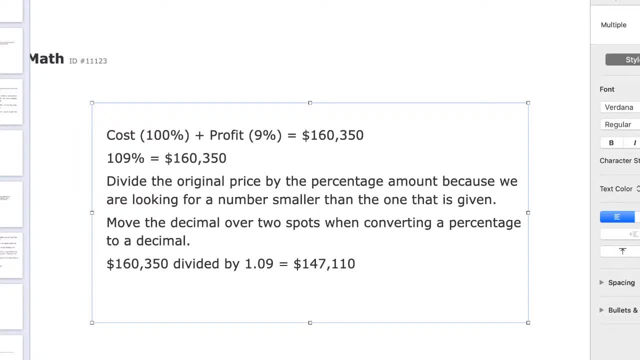 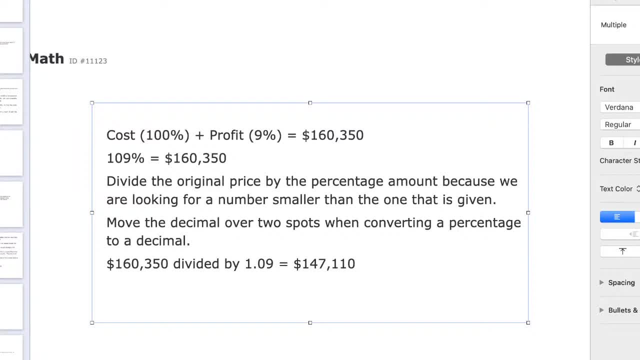 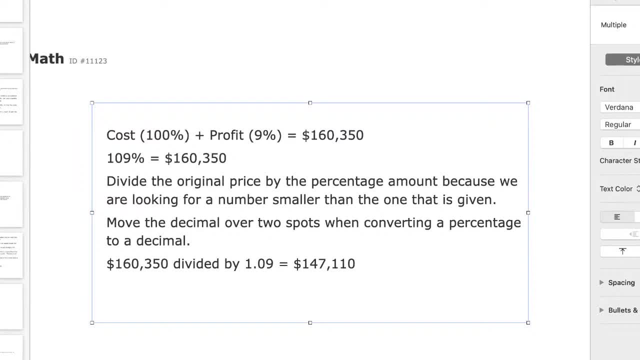 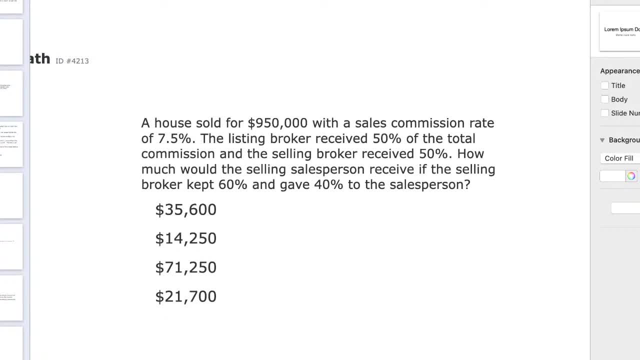 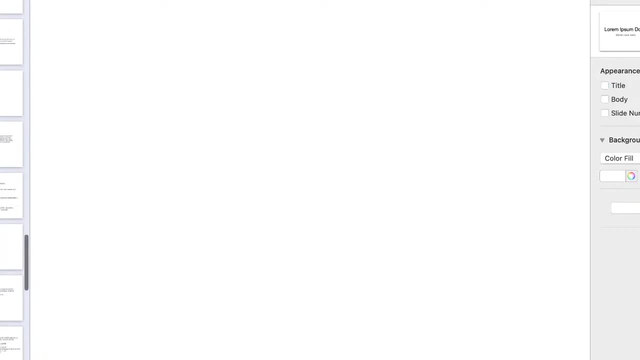 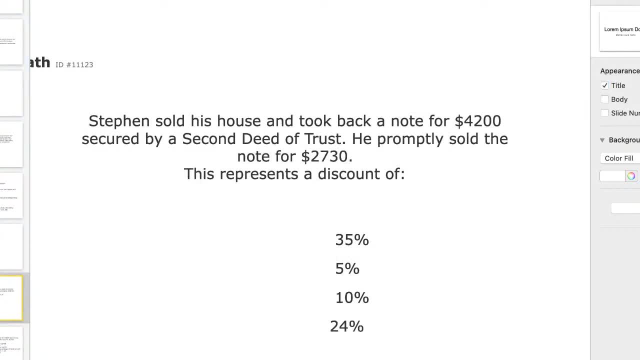 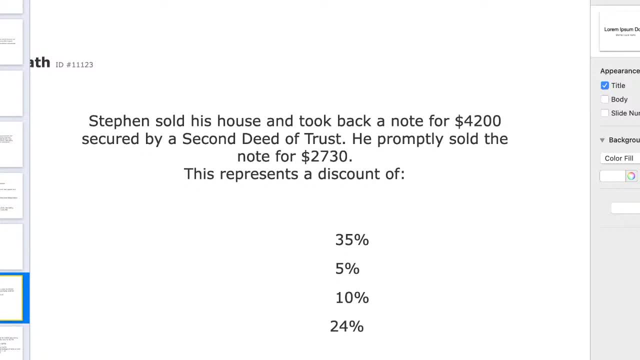 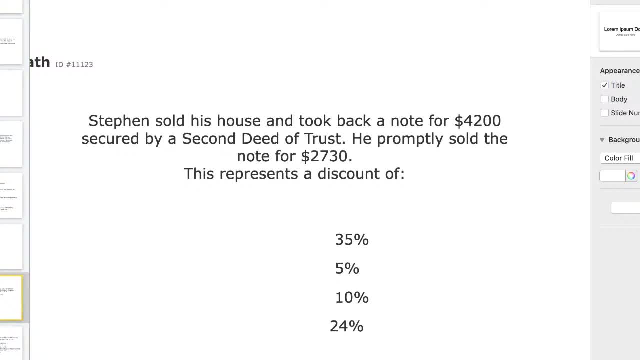 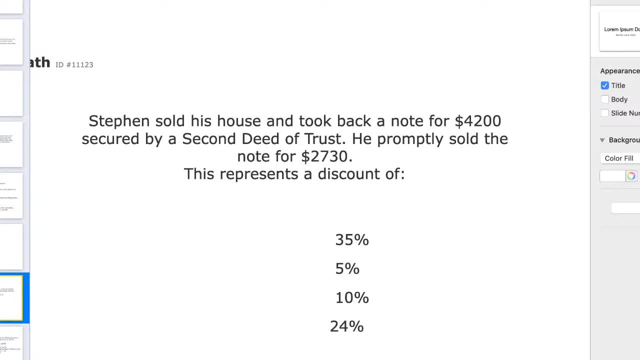 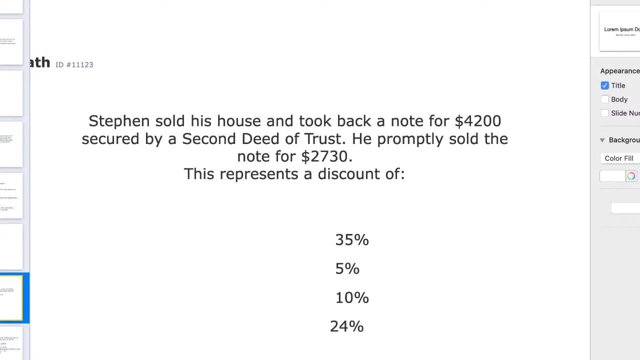 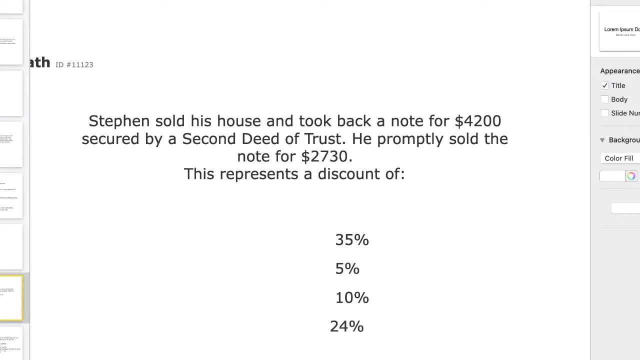 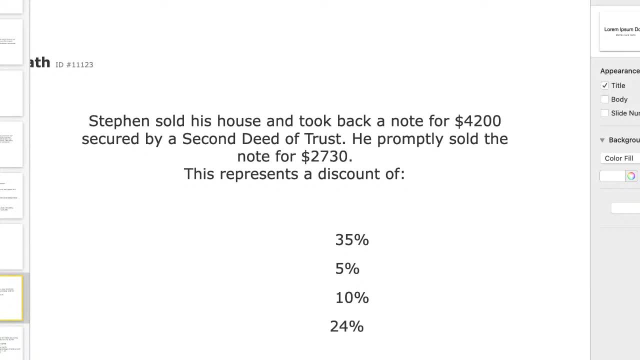 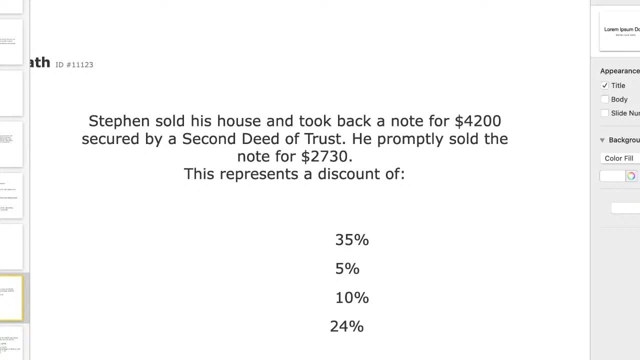 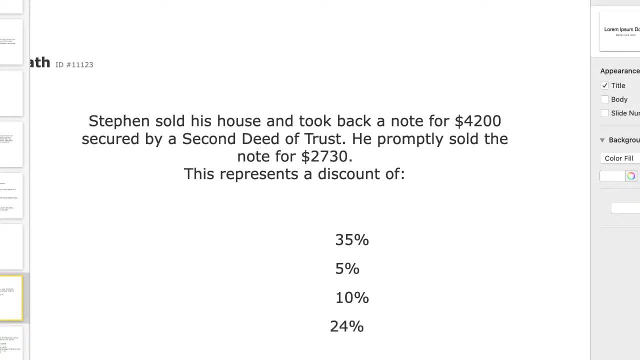 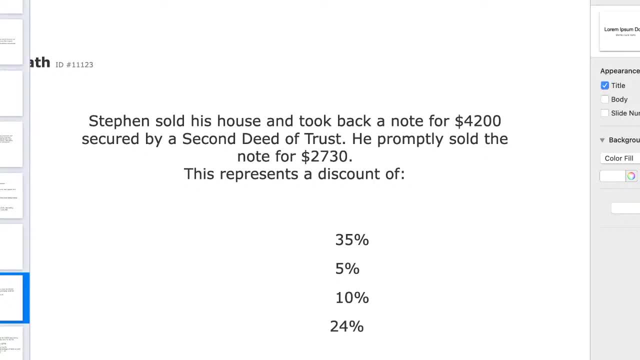 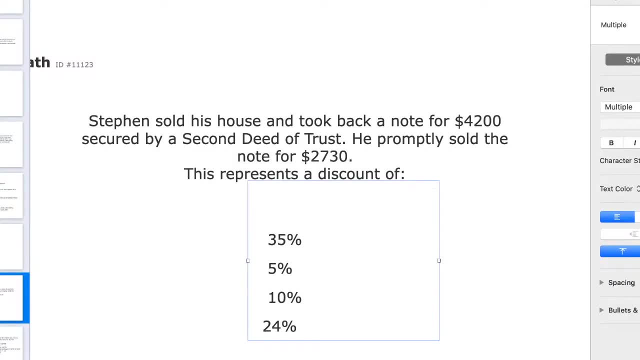 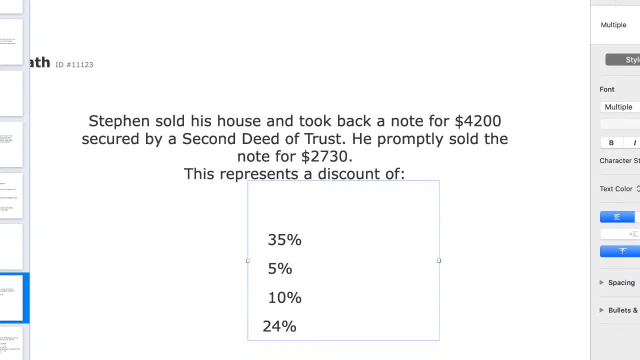 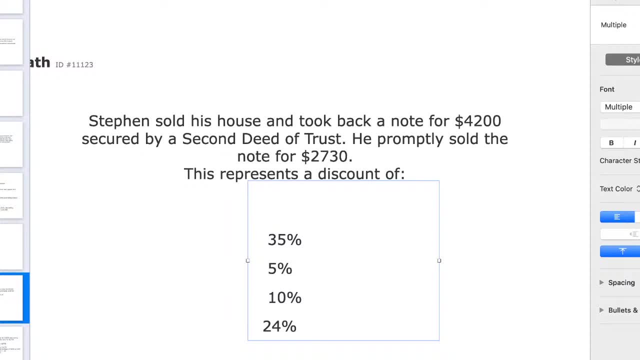 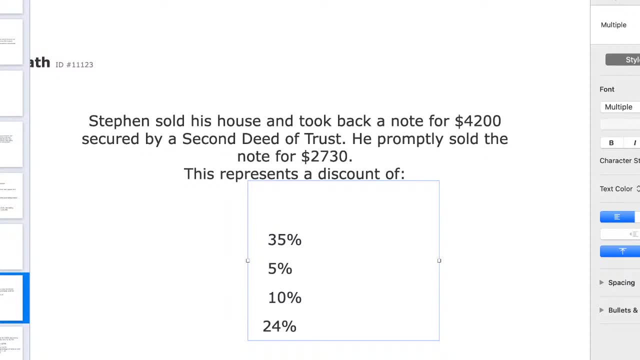 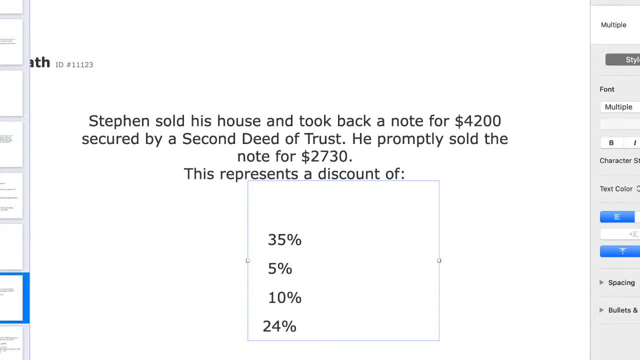 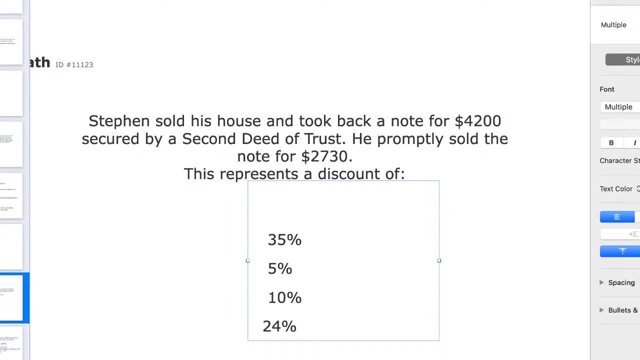 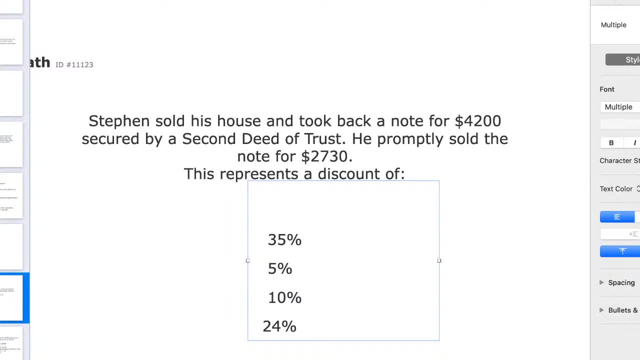 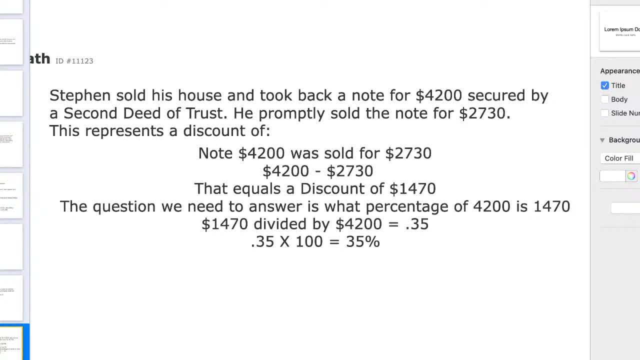 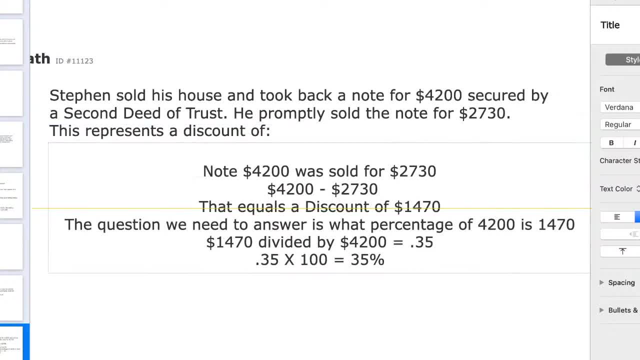 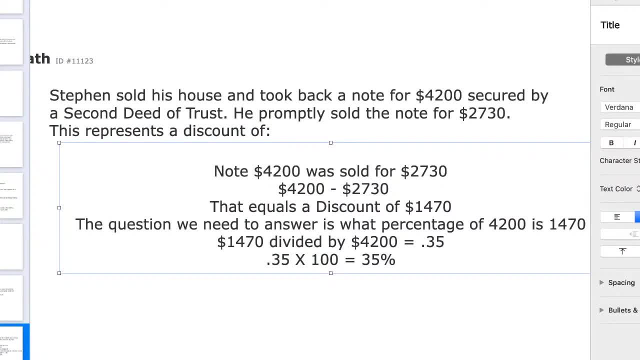 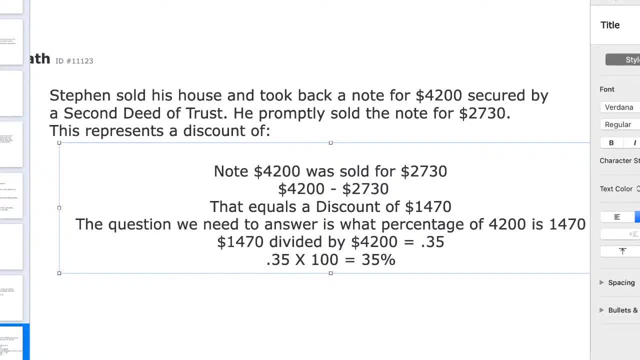 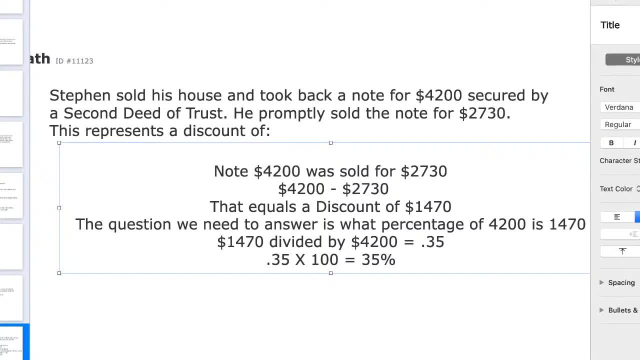 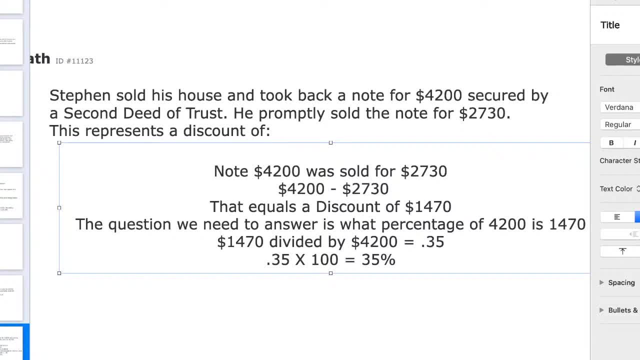 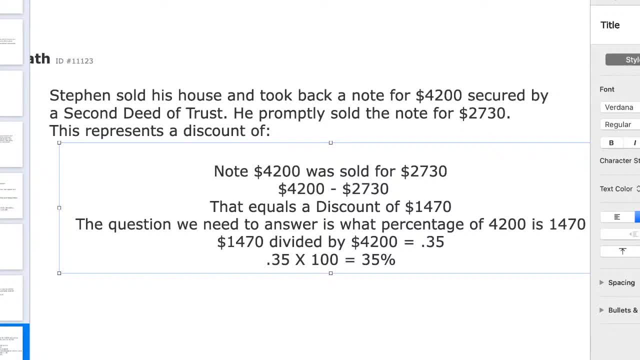 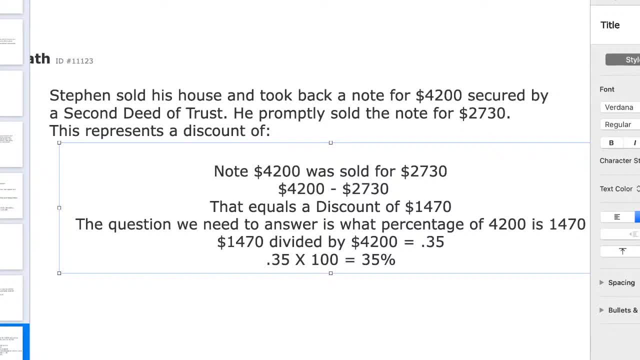 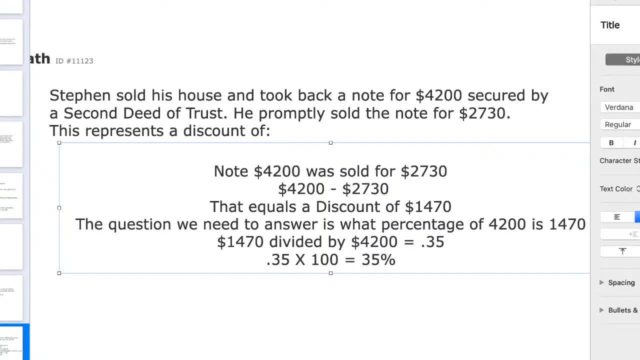 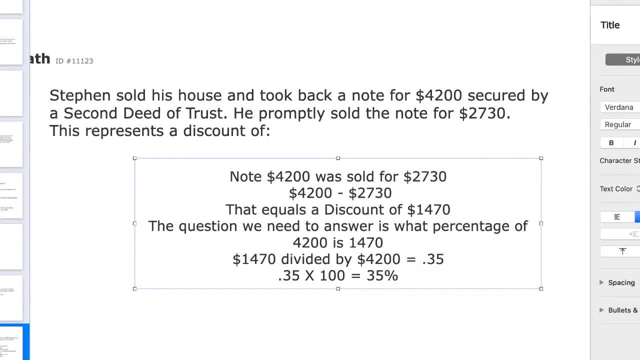 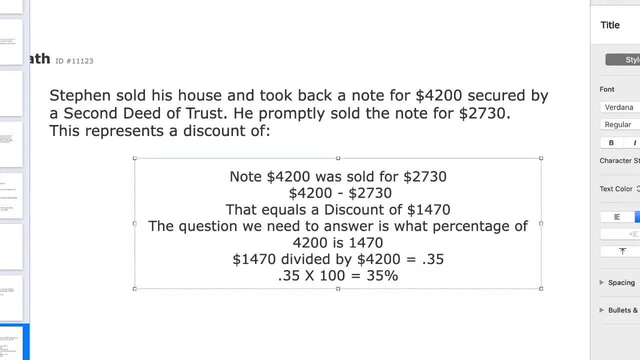 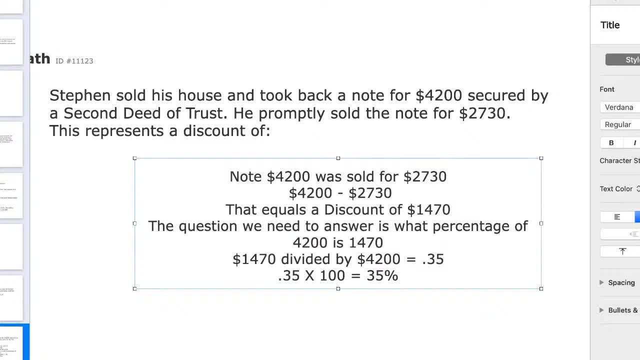 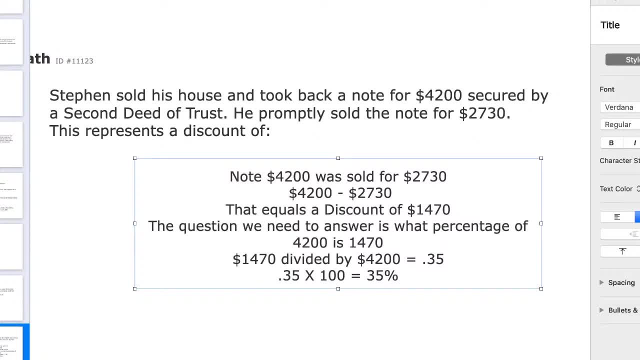 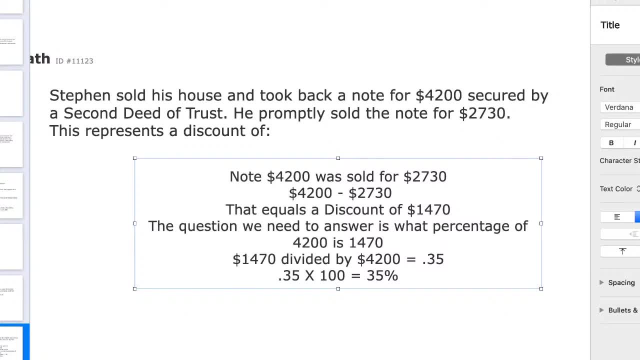 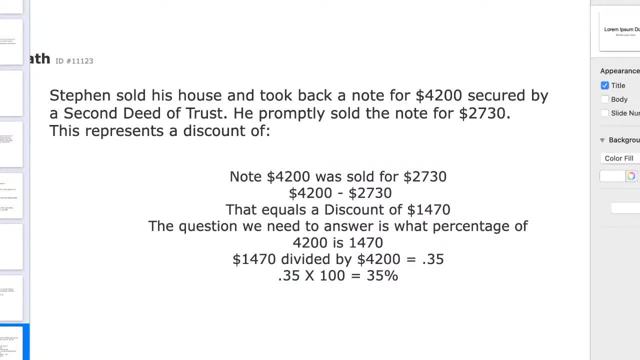 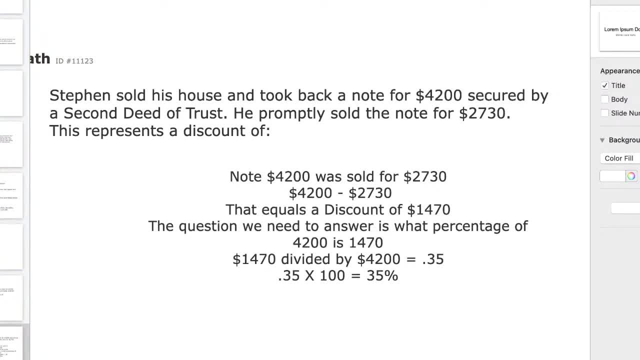 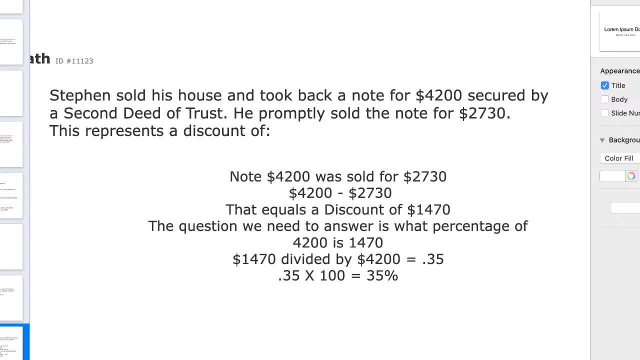 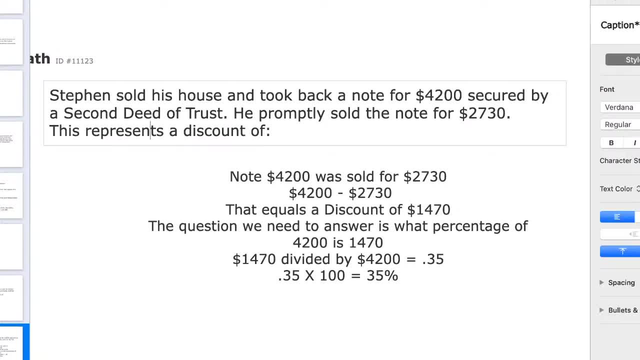 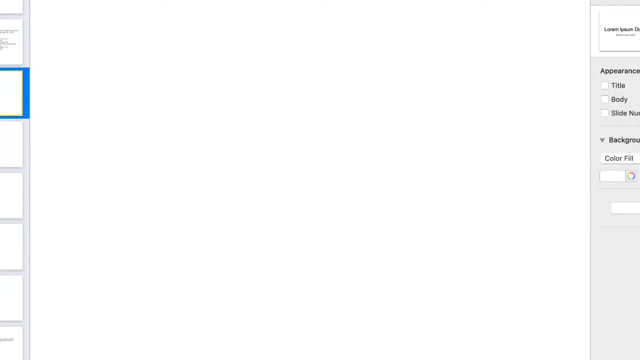 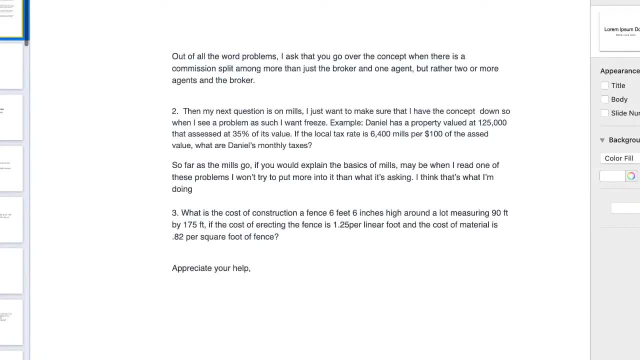 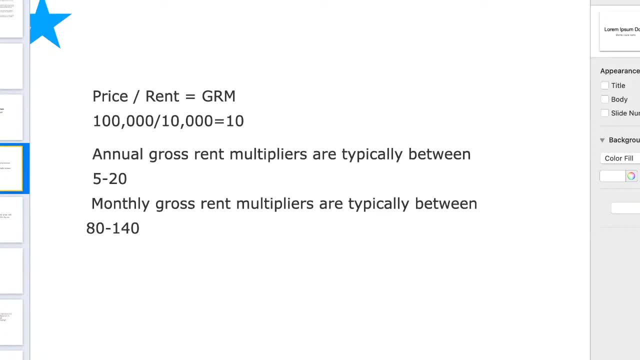 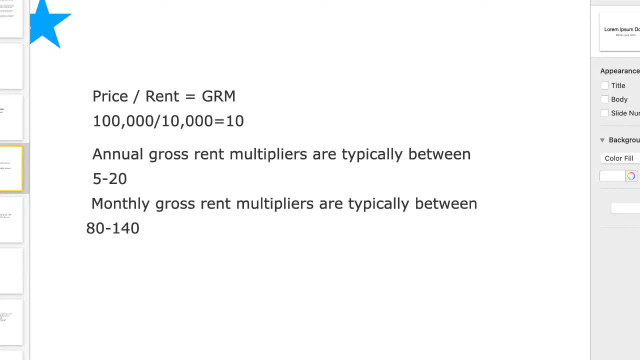 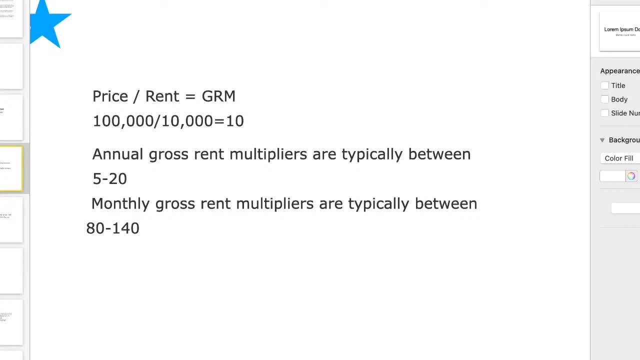 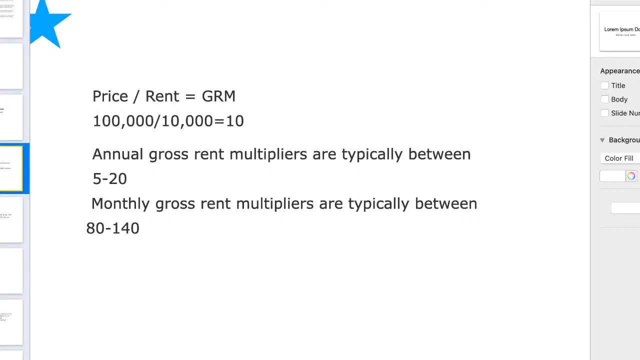 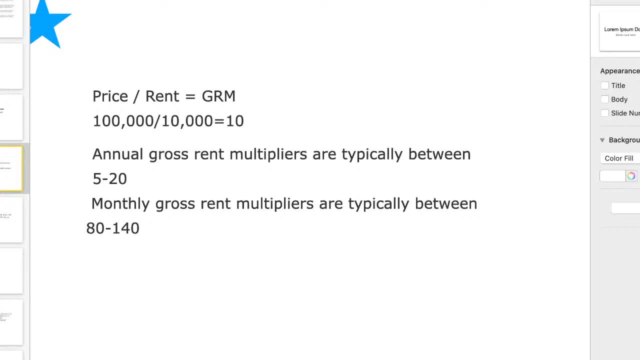 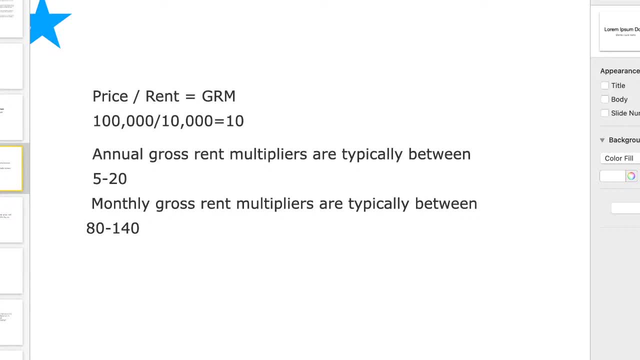 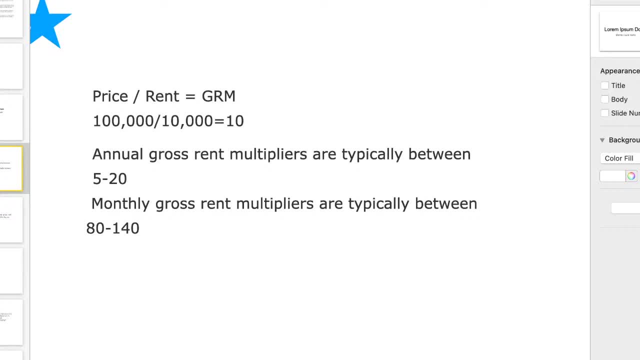 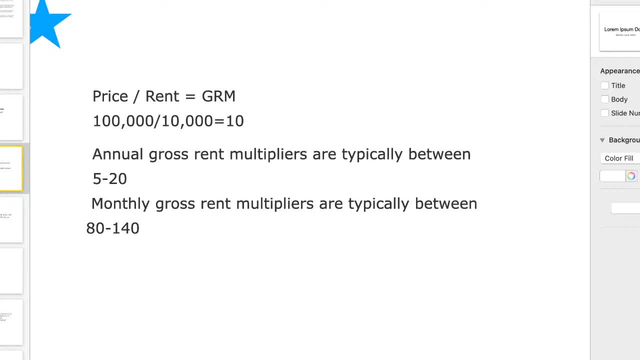 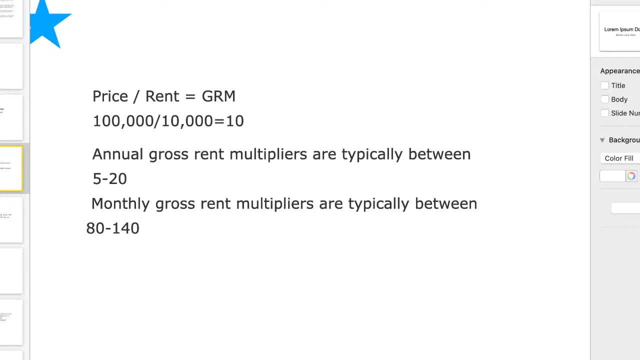 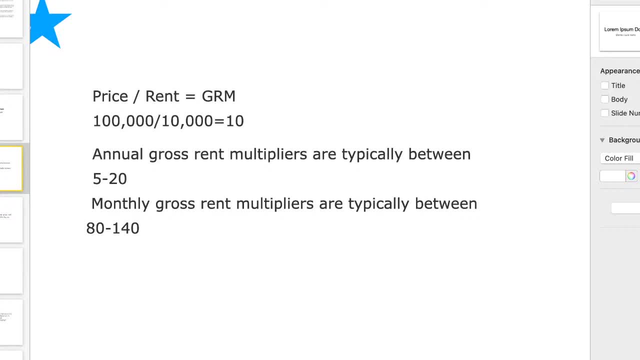 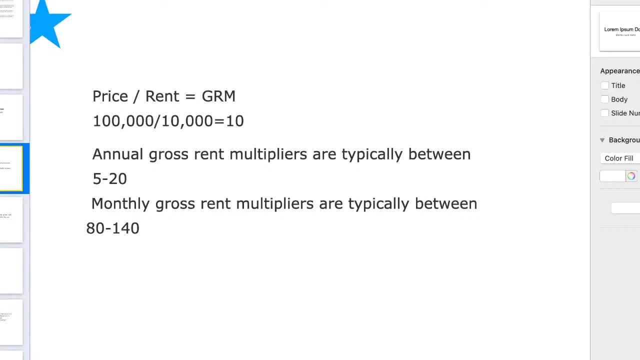 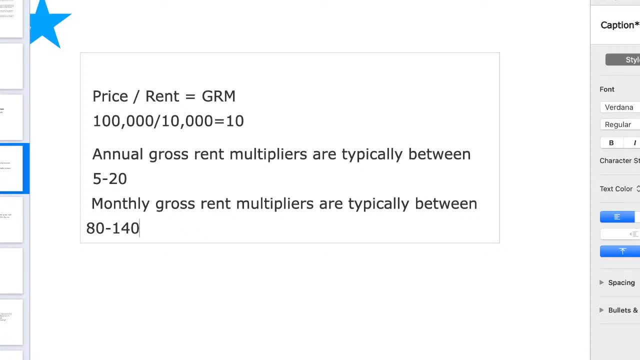 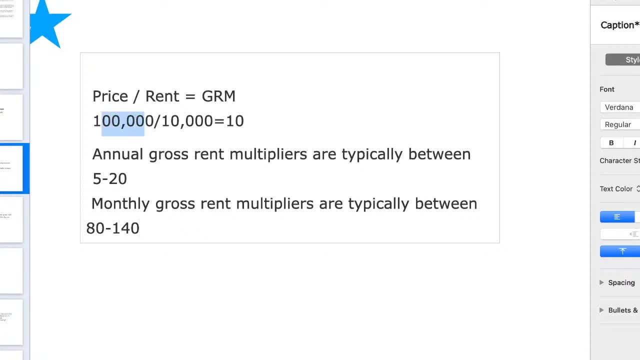 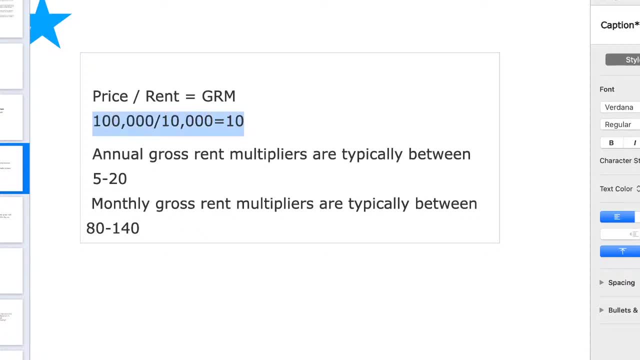 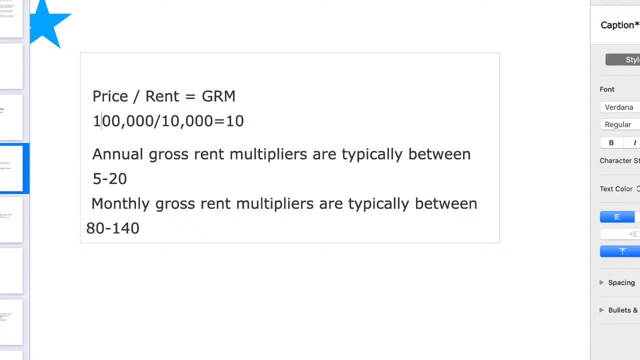 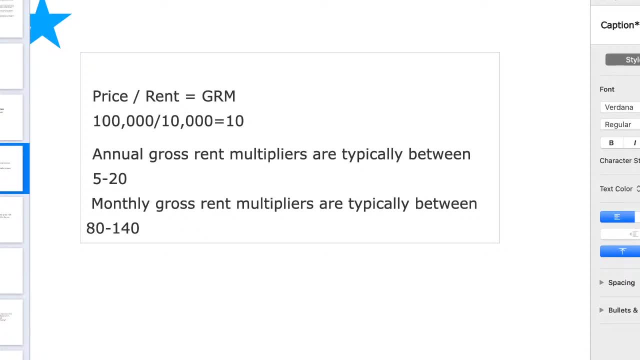 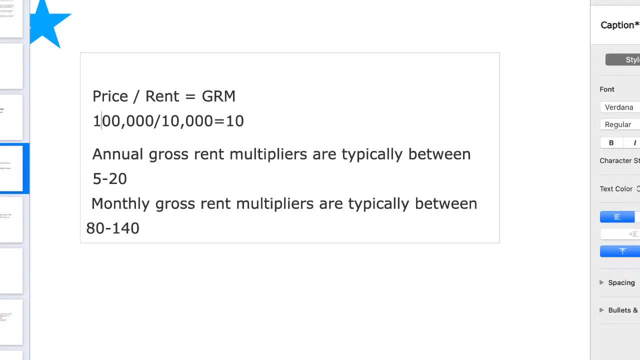 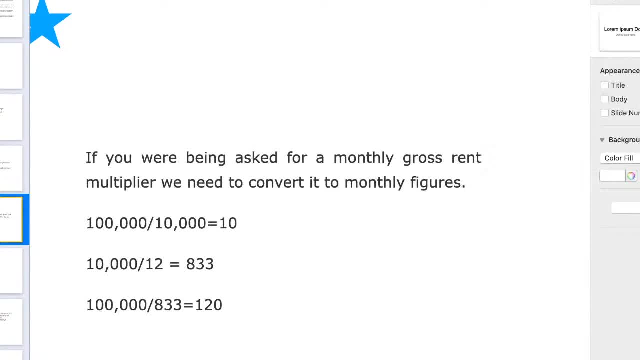 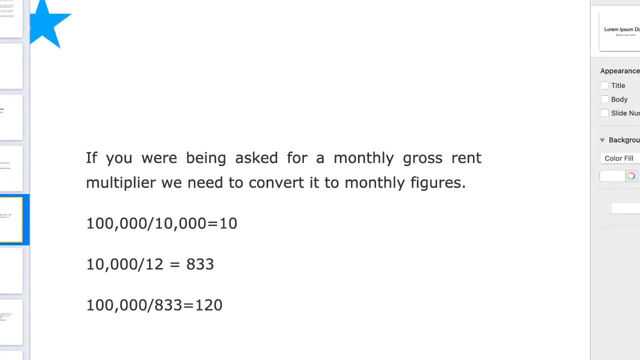 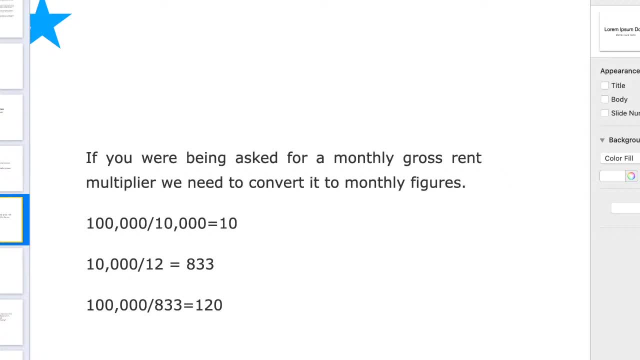 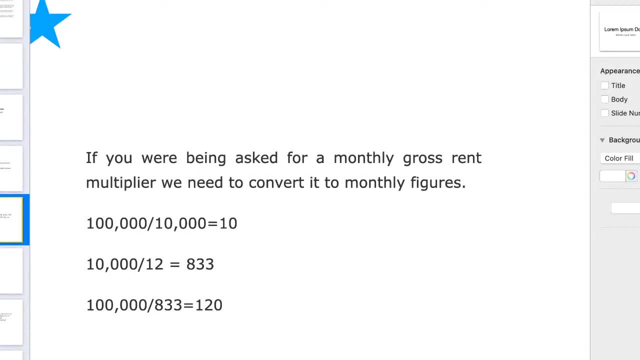 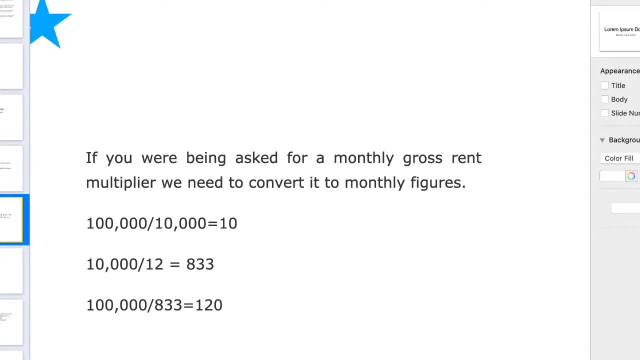 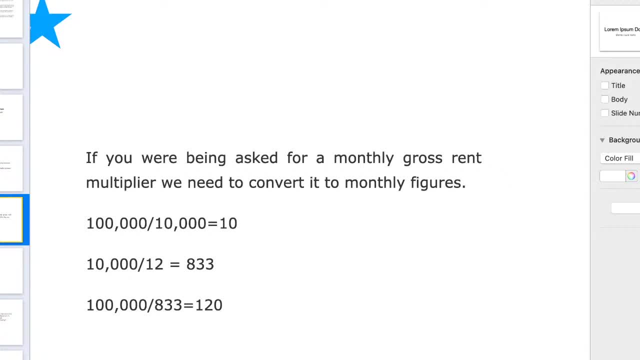 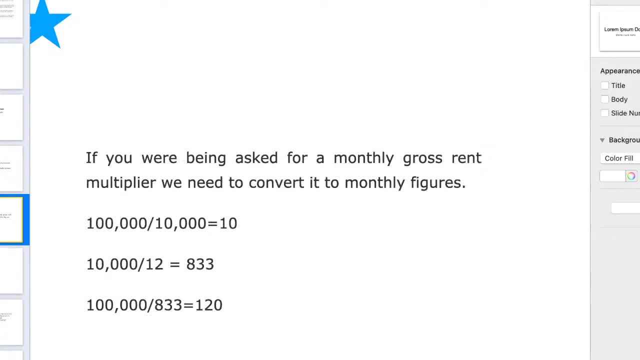 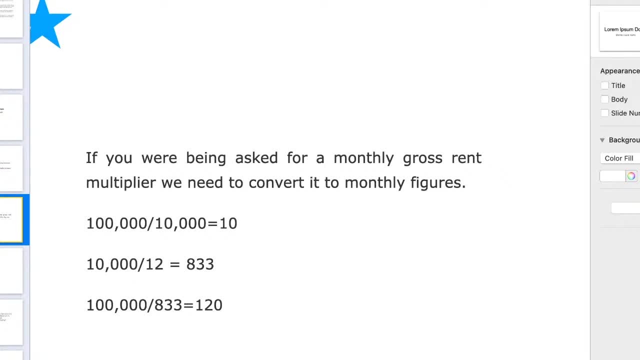 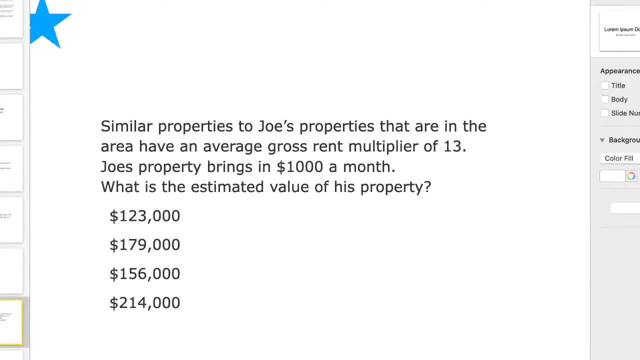 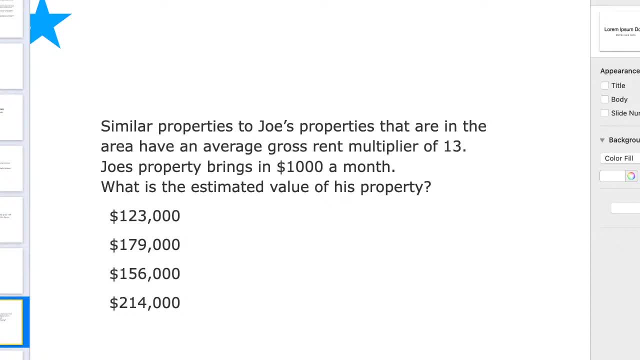 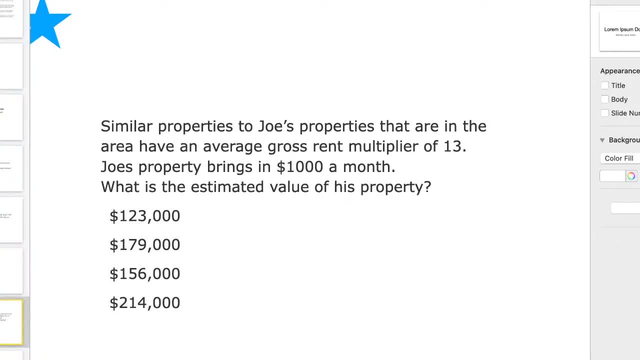 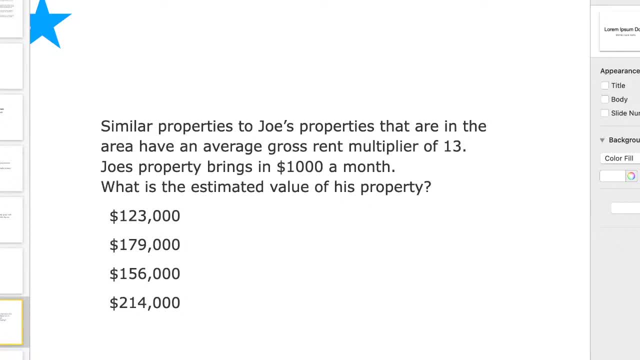 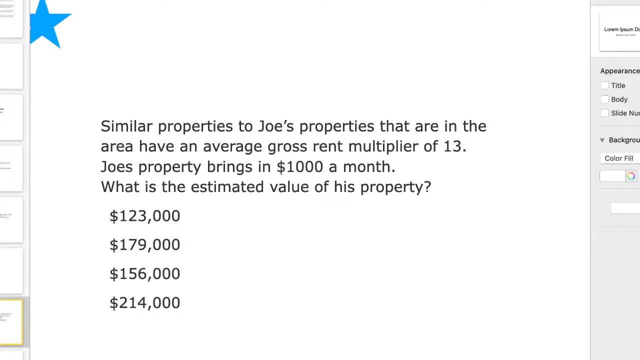 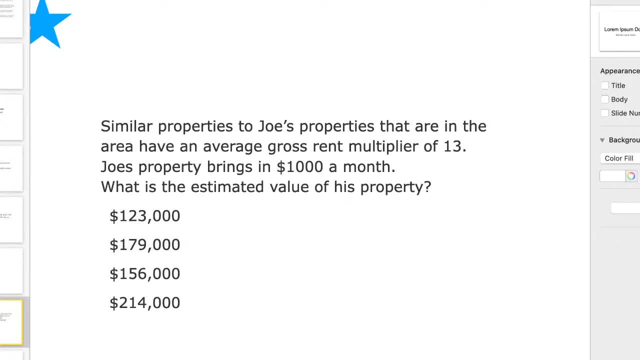 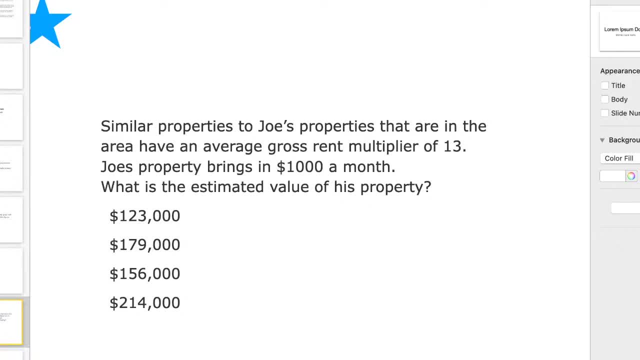 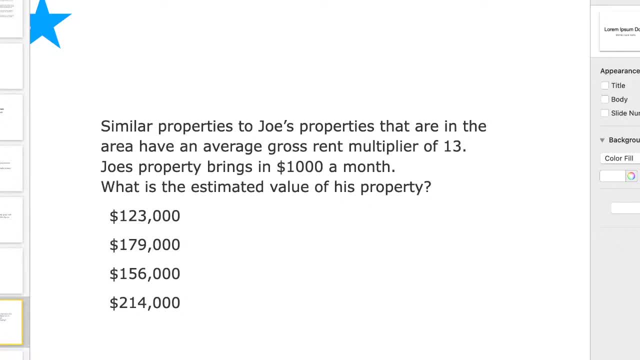 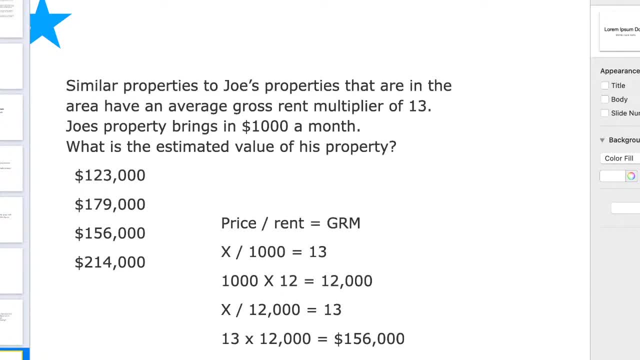 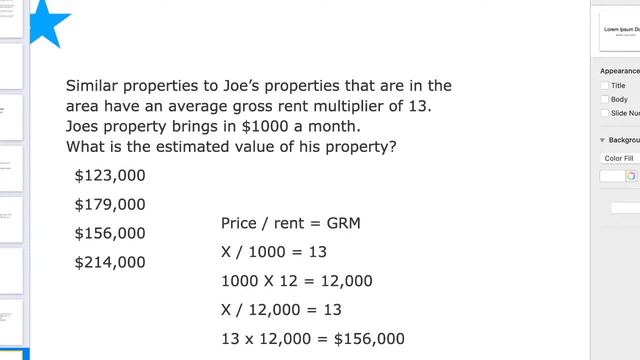 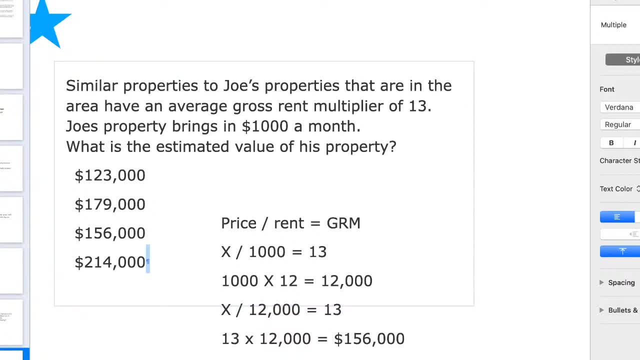 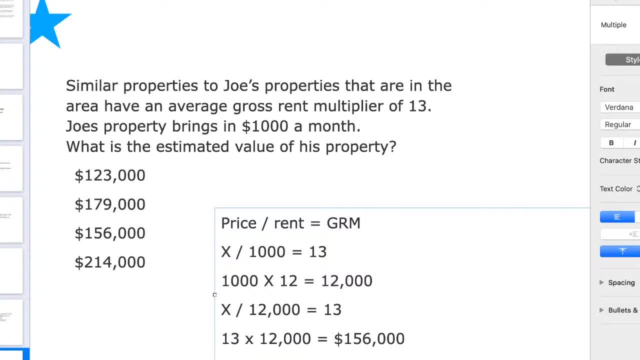 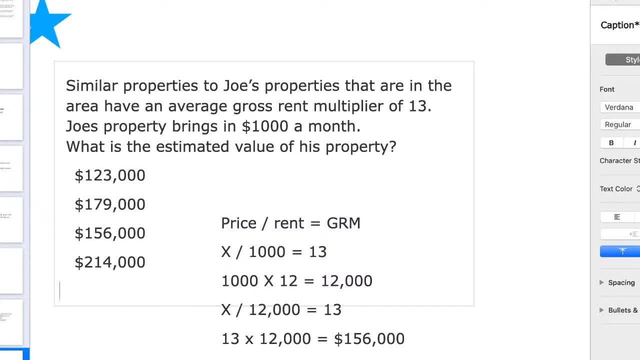 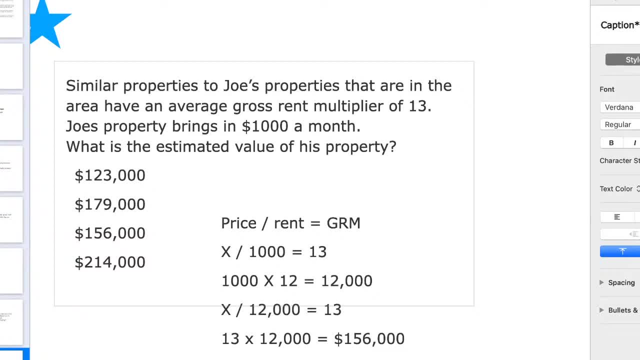 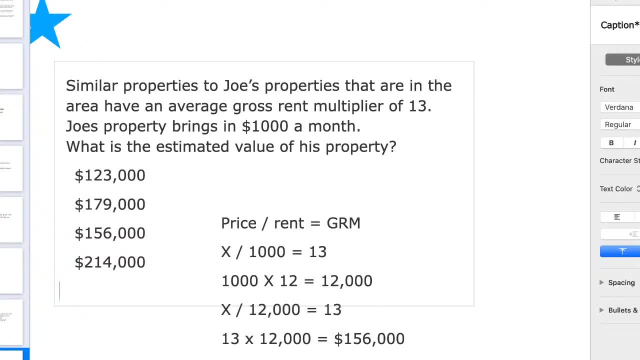 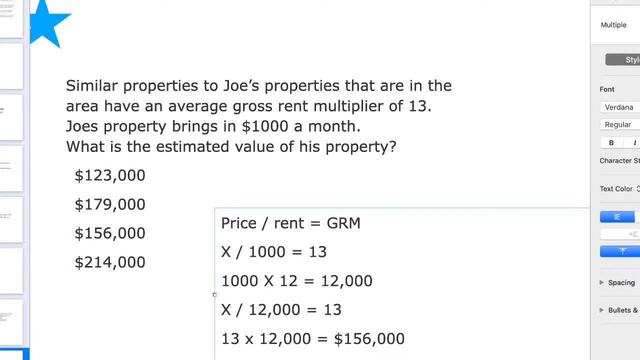 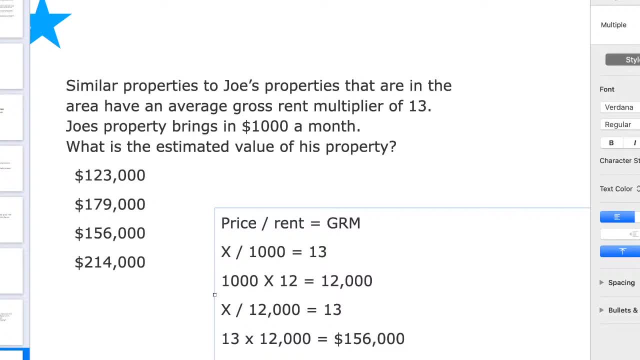 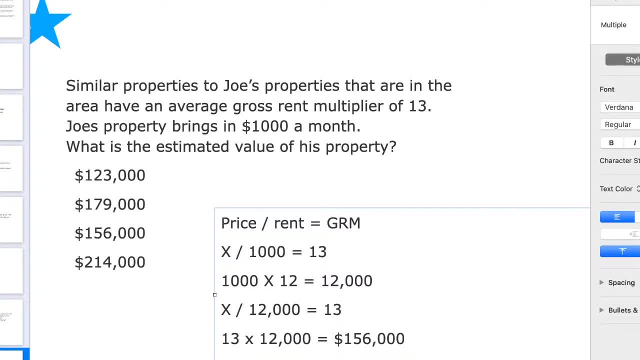 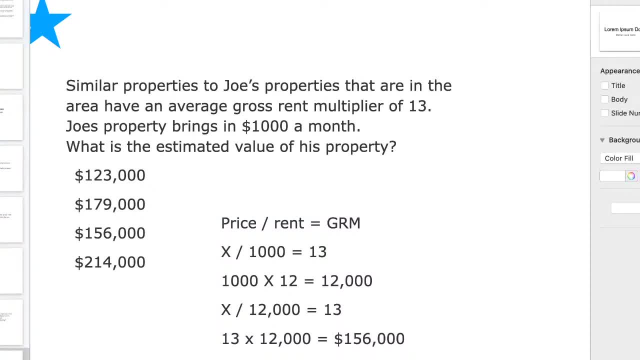 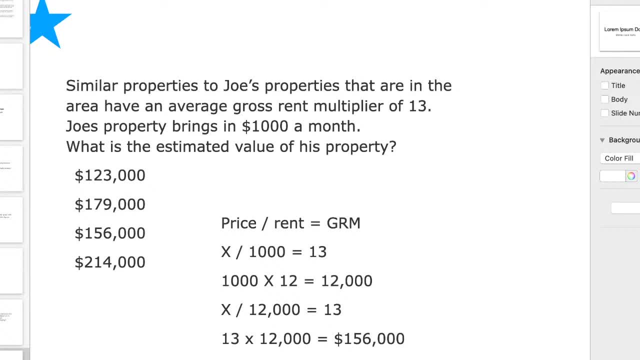 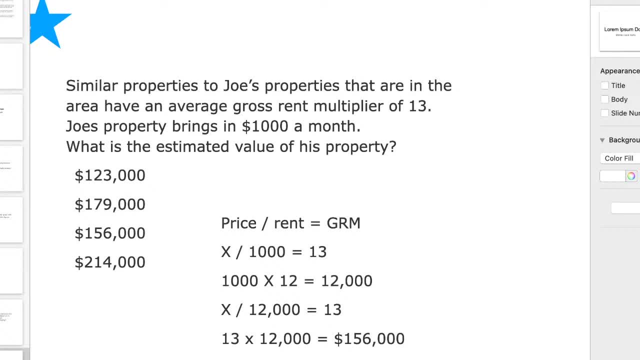 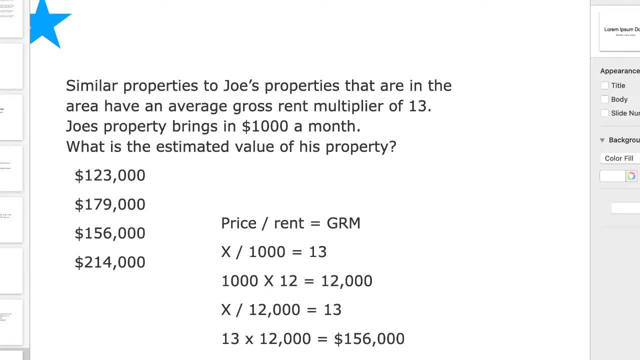 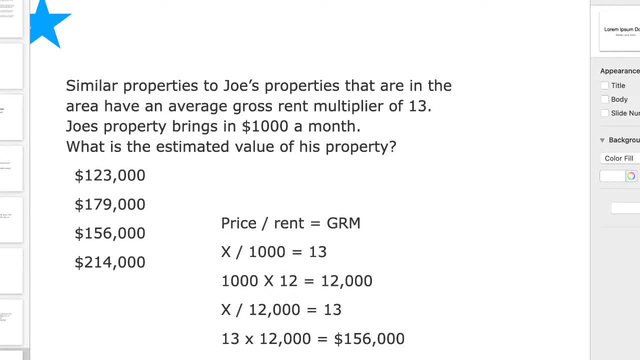 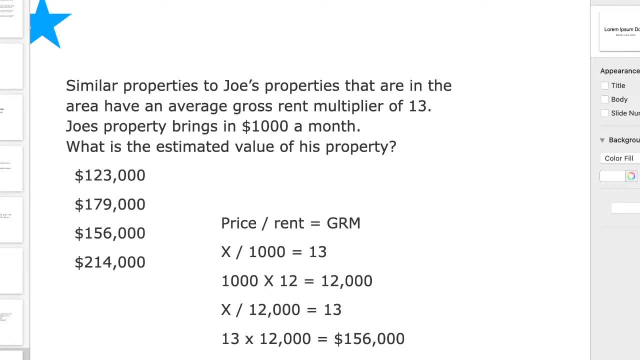 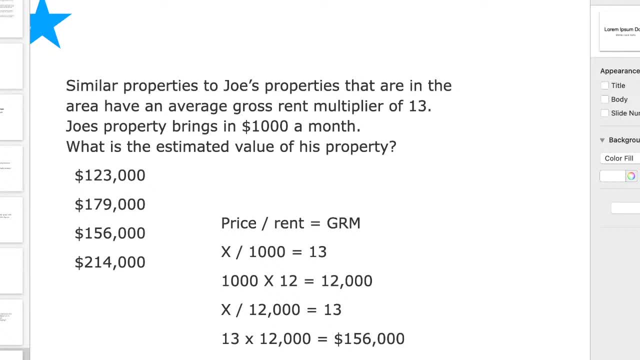 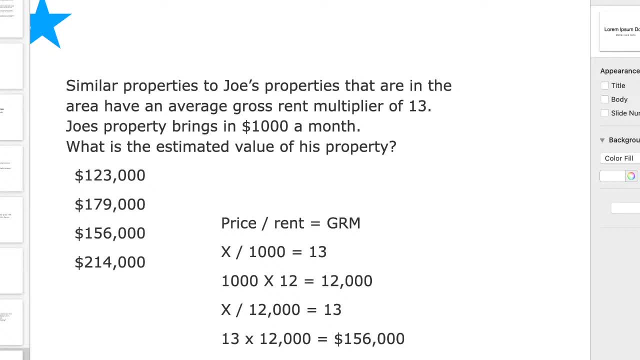 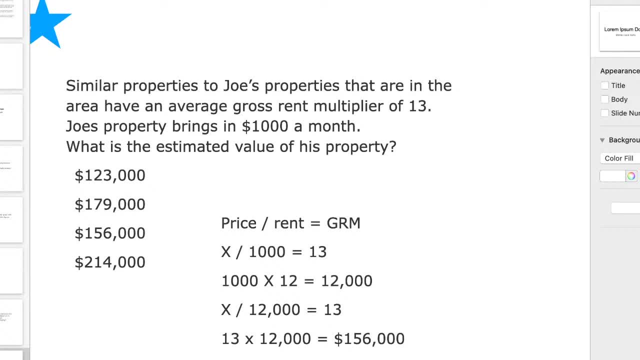 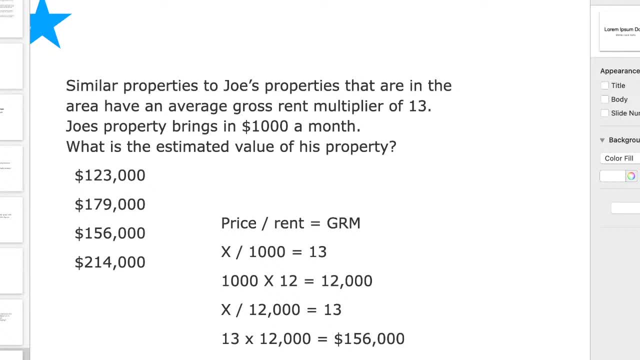